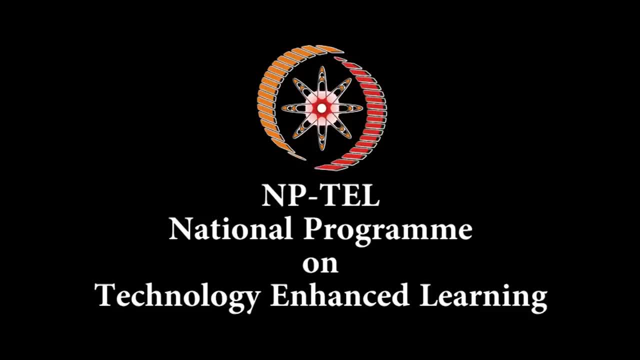 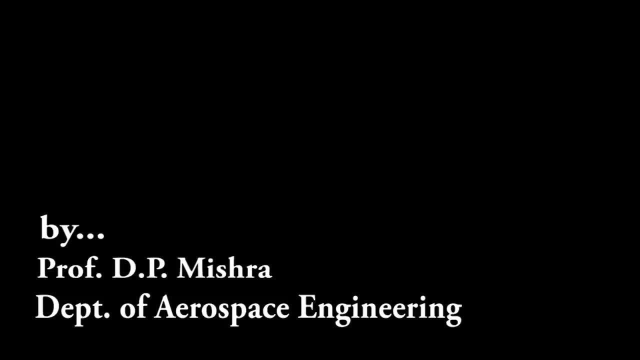 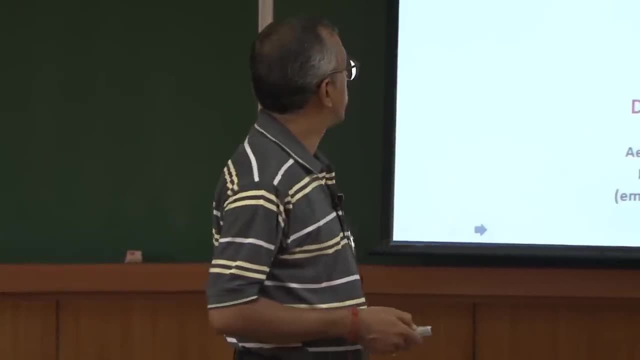 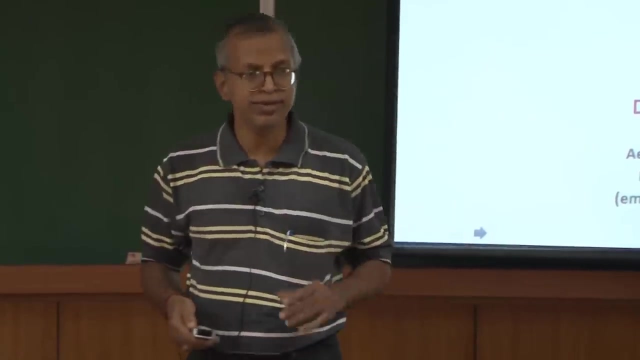 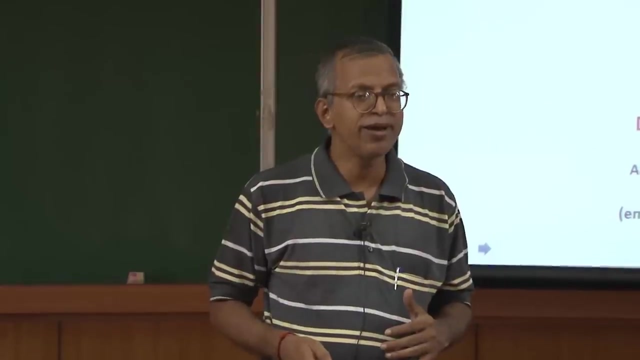 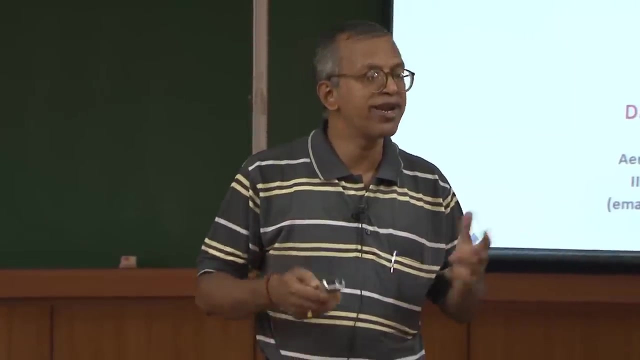 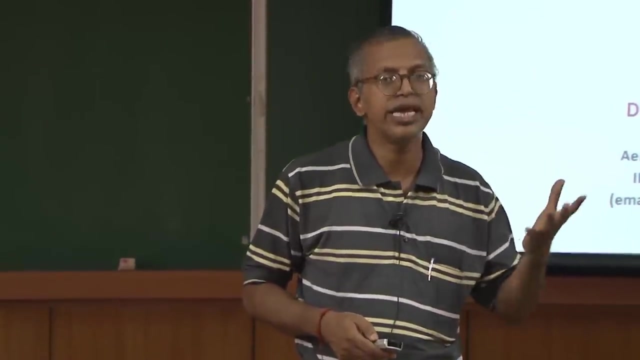 I welcome all of you to this course: Fundamentals of Aerospace Propulsion. And if you look at an open sky, whether during the night time or in the day time, you will be wondering what really it contains, Am I right? All of you will be have a wonder how it is If you. 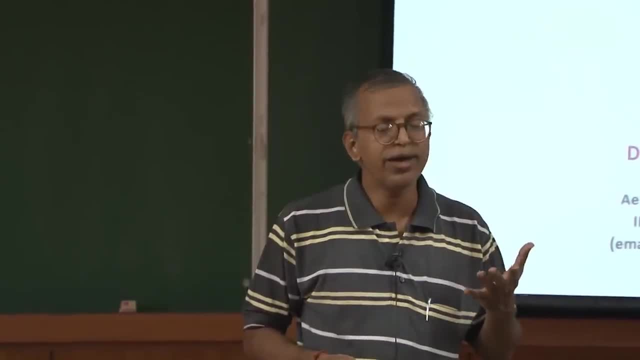 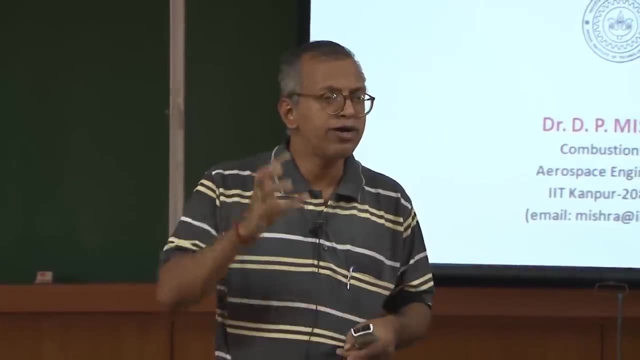 look at a sky in the night time, particularly in the day time, you will be wondering what it contains. If you look at a sky in the night time, particularly dark, pitch night without any cloud, you will see that lot of stars will be twinkling at you, Whenever I 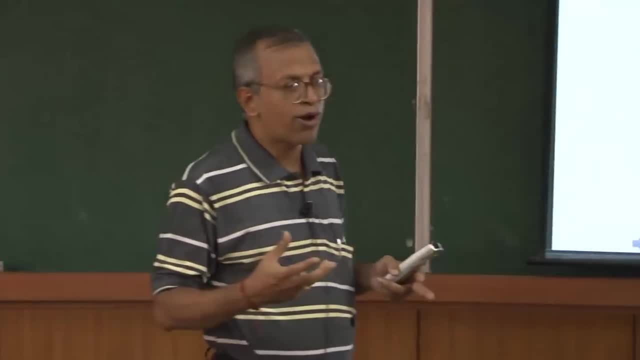 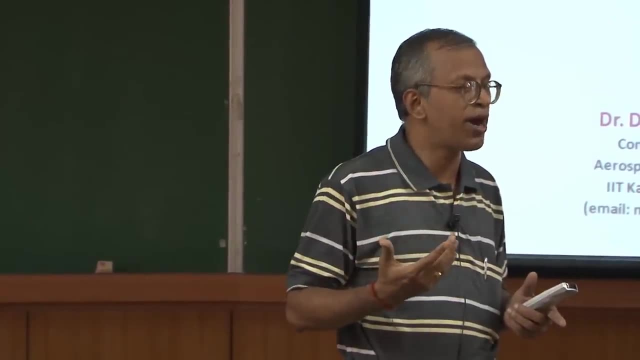 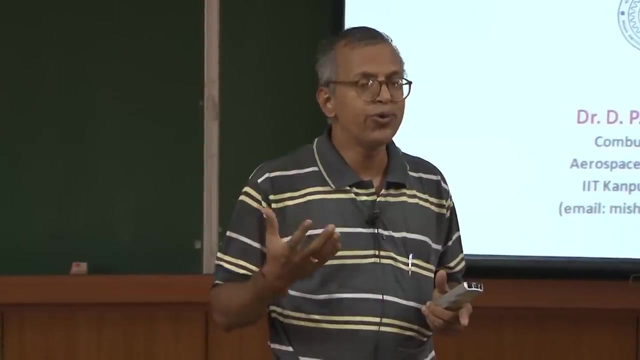 see that I remember a song- twinkle, twinkle little star, how I wonder what you are. And that still is remaining in my mind from the childhood And I hope, and I am sure, that lot of you will be having similar feeling. to look at what it contains, 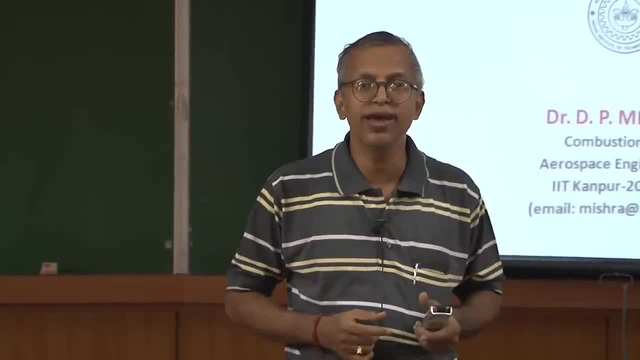 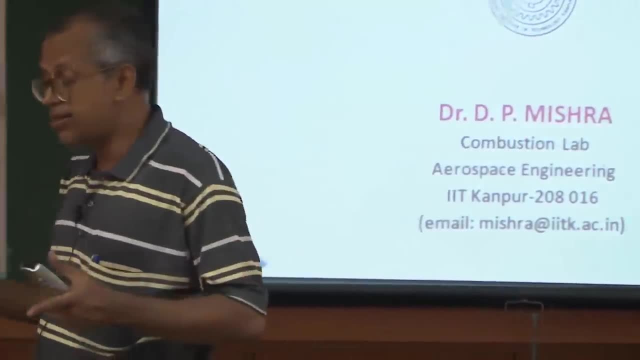 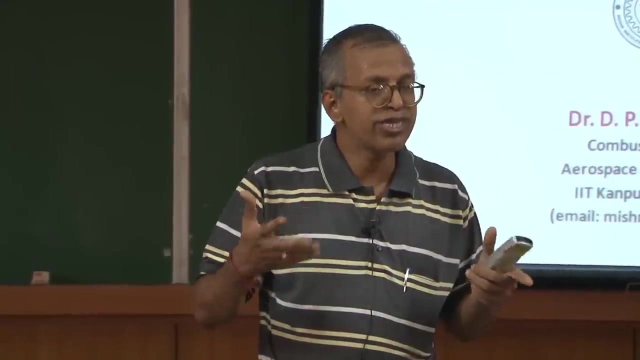 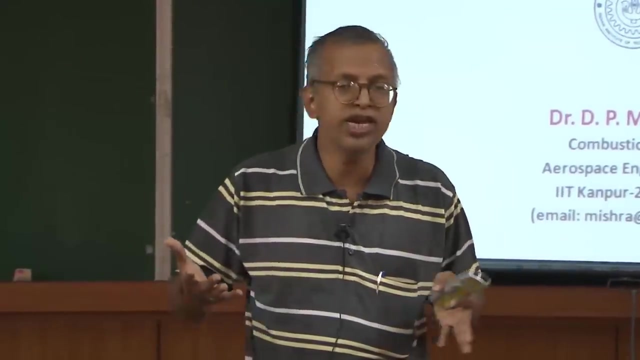 Why it is twinkling. How many stars will be there? Can anybody tell me how many stars will be there in the sky? There are 200 billion galaxies. according to the scientist estimation, as of now, One galaxy will be containing something 300 billion stars, And we are in a galaxy. 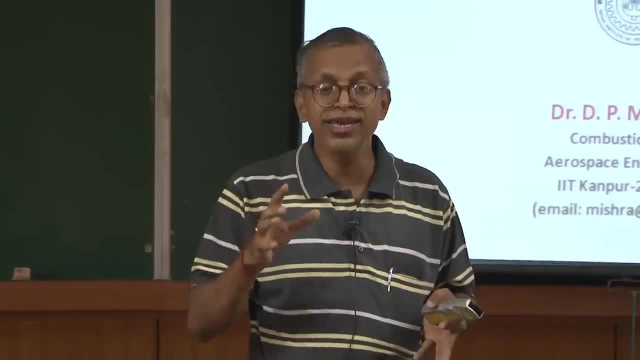 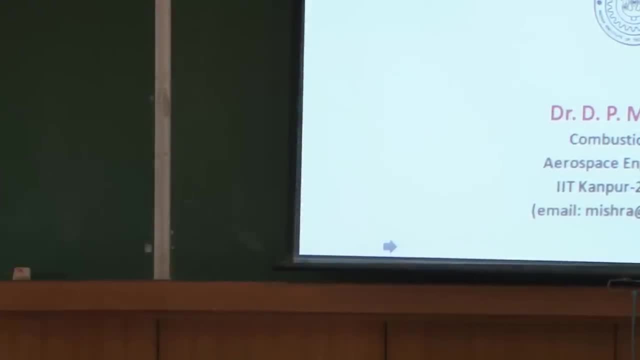 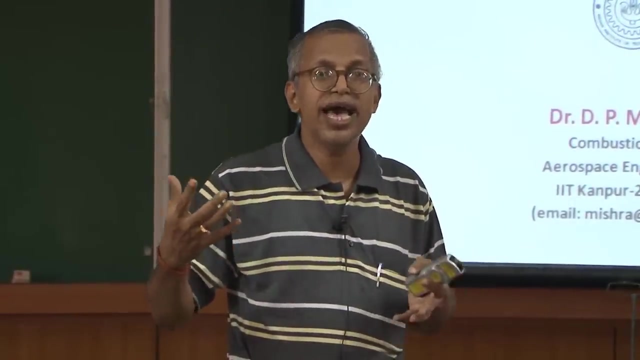 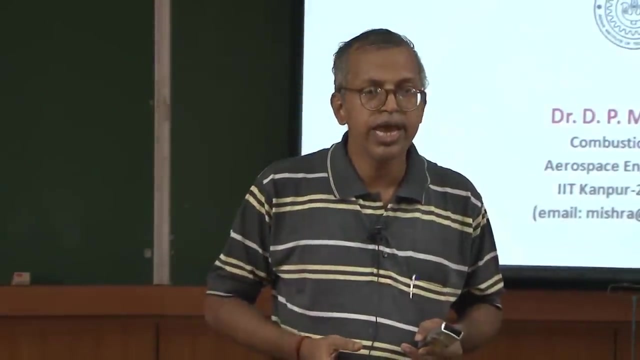 known as milky way And where sun is the one of the star. we support all our- you know- energy requirement. all the life in this solar system, And this, if you look at always, man is has a desire to look at wonders and how it will understand the thing, And this is. 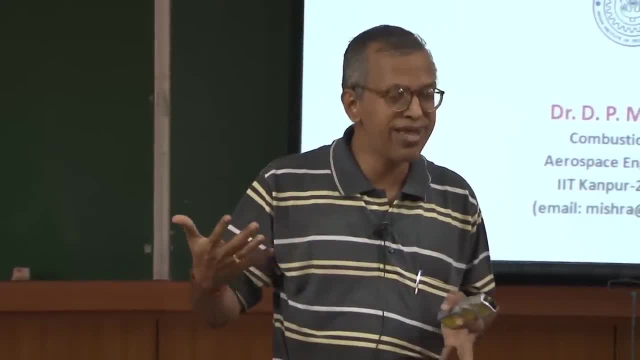 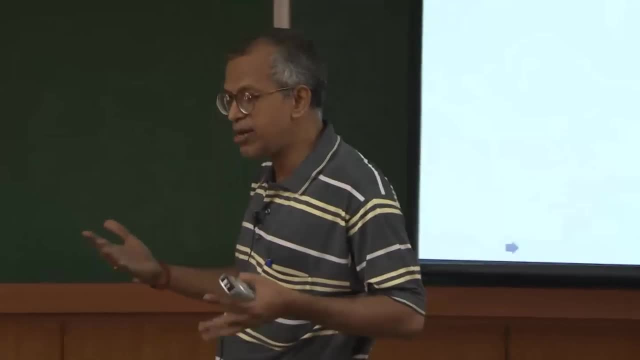 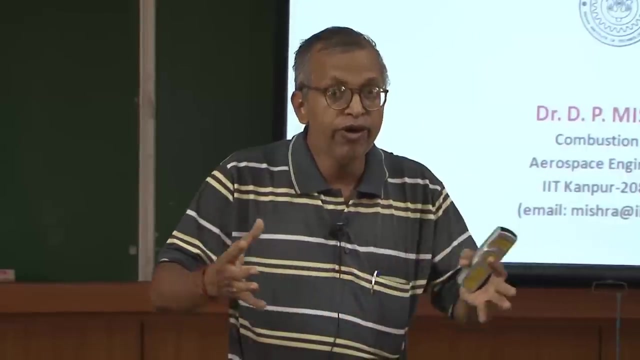 a revelation due to the development of the solar system, Science and technology. do not think that this modern scientist have found out this. This was there in our scriptures also about very exact next of that, Like, for example: people were thinking: the whole universe is expanding. one day it will contract. That is nothing. 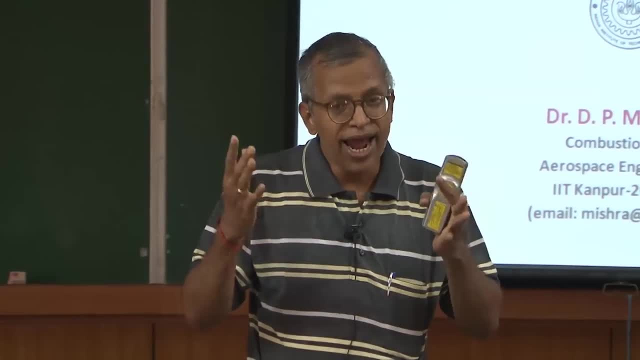 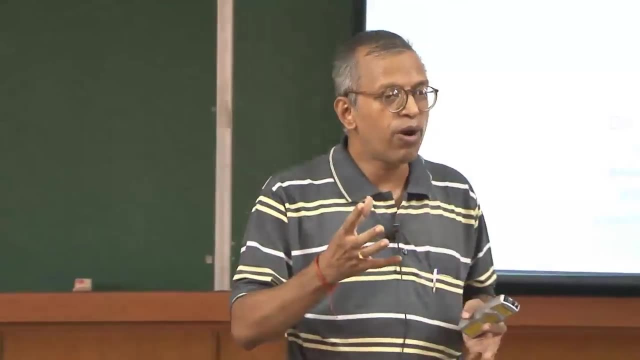 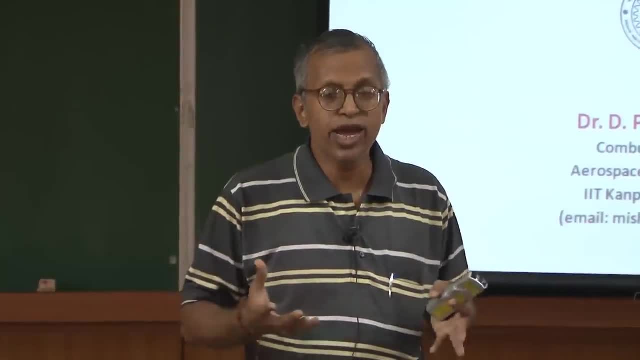 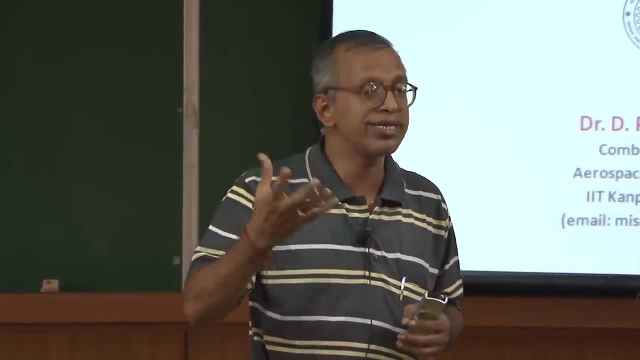 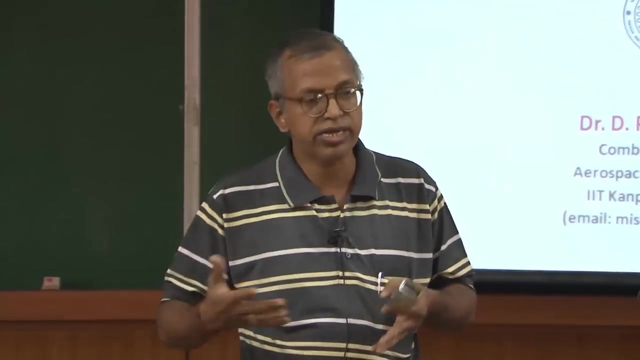 How to move about it. How to move about it If you look at it like today. we are in the moon mission. India is having a very prestigious moon mission- How to move about it? How to go to a moon and sea? And so also there are planetary missions of USA and USSR and China. 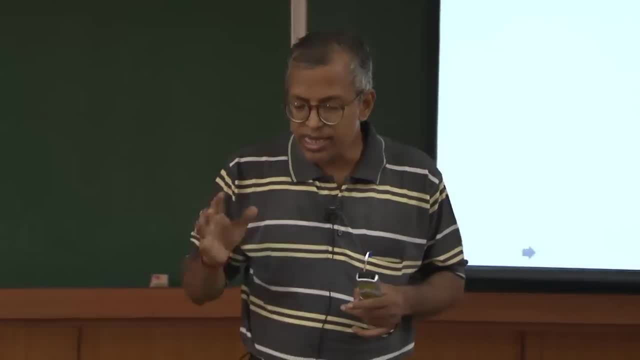 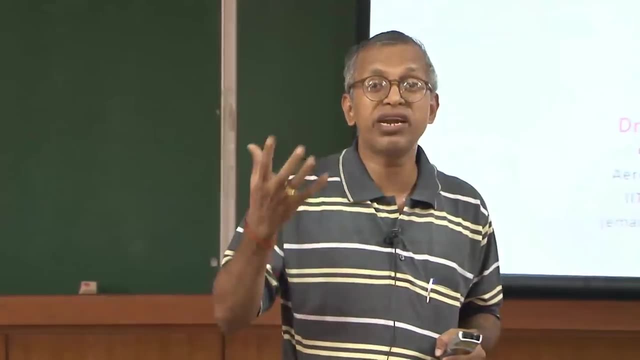 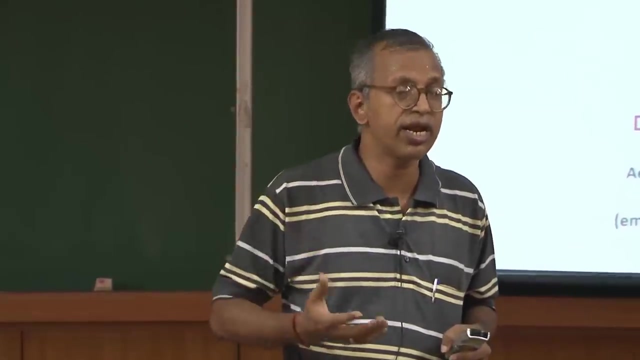 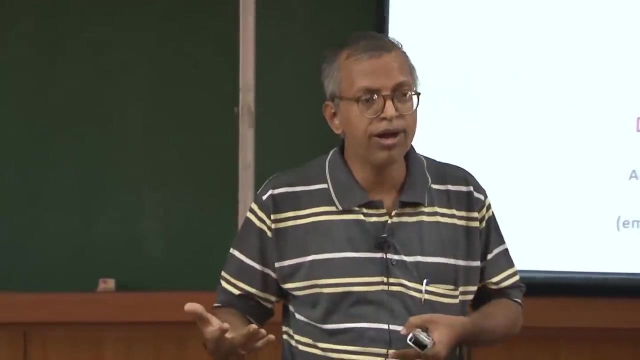 and several other countries. Now this has motivated in Offlet to look at how to have better propulsive devices such that we can, you know, meet our requirements. and beside this there are several other application, like satellites and others, which will be helpful not only for the winning a war but also for civilian applications. 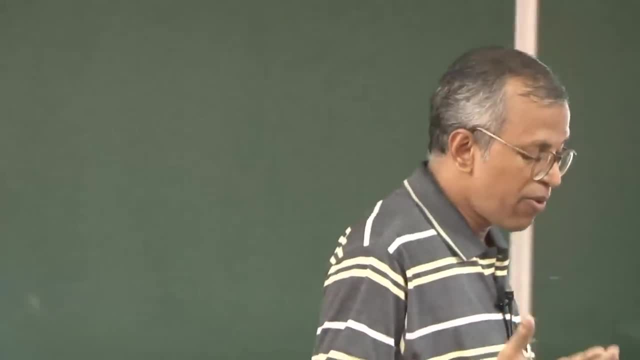 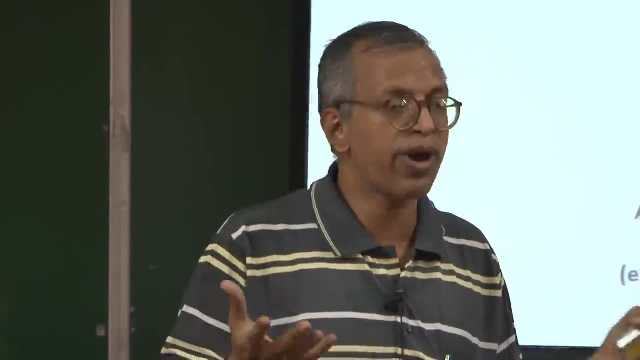 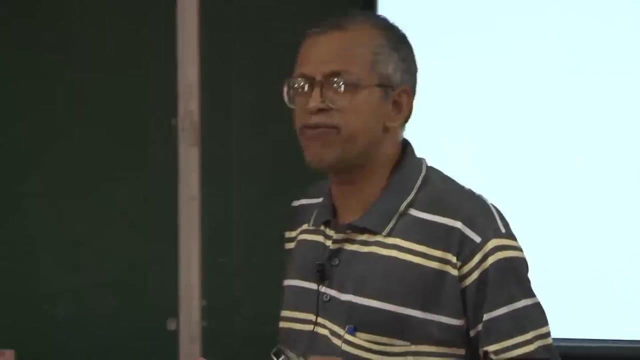 And besides this you might be knowing, you might be wondering how one can really fly, because whenever I see in this beautiful campus of IIT Kanpur birds, I always feel how they fly, and this kind of questions comes to the mind of the ancestors from the time immemorial. 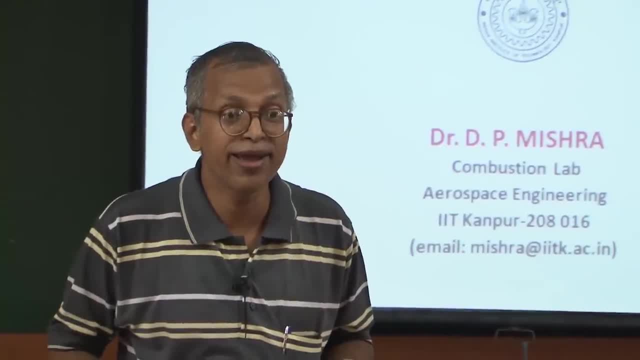 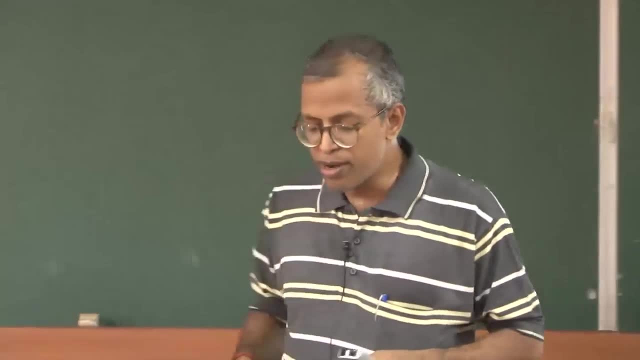 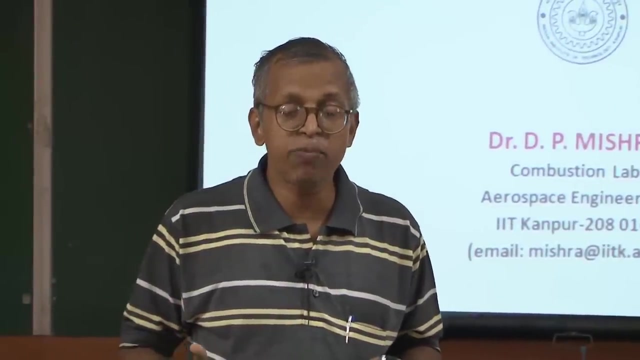 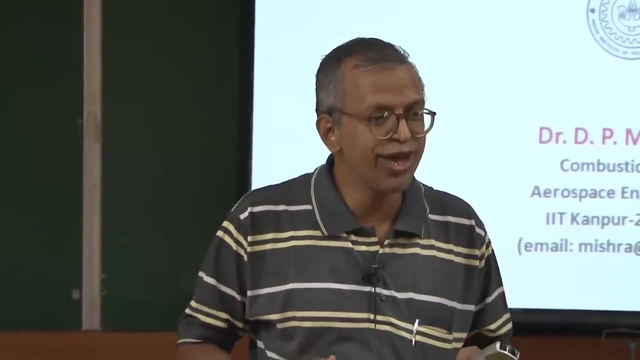 that: how does a bird fly? Can we not fly like a bird? and there are several stories. I will tell you a story, what my grandmother had told me When I was a child. she told me that my great, great great grandfather had attempted to fly like a bird. whether it is a story or a reality, I do not know, but it was being placed on. 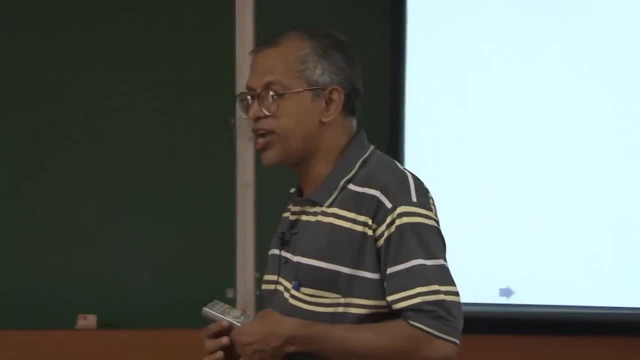 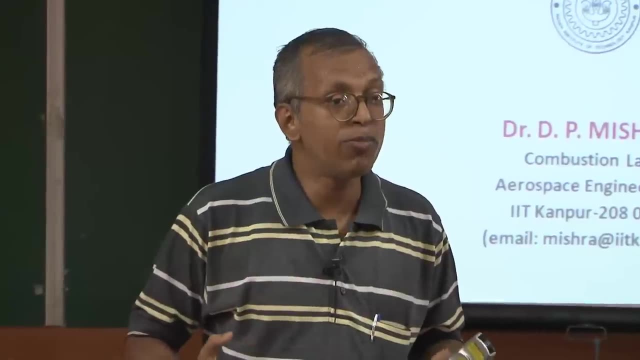 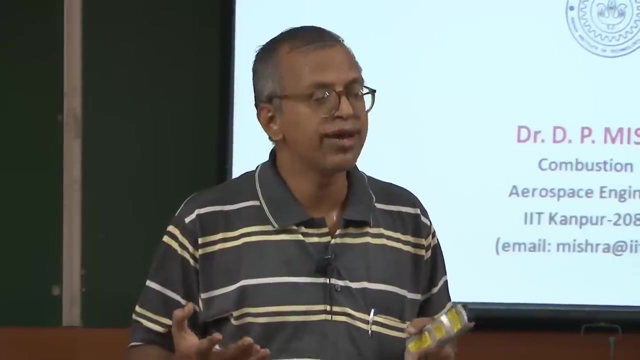 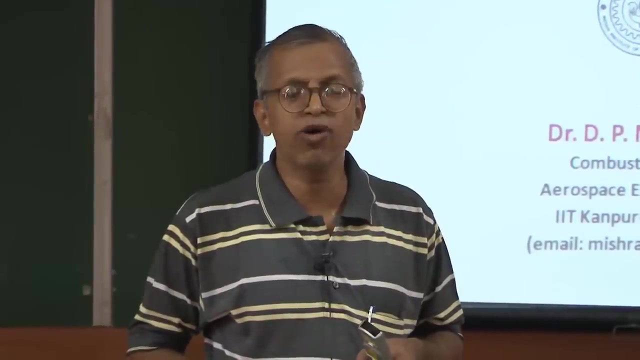 me as a reality. So who was trying to strap a wing to his very arm, made out of bamboo, but unfortunately he made And accident which was killed him in the process. that is why it became a story, And similar stories you may find in our mythology, studying from Hanuman to Jambavan and several. 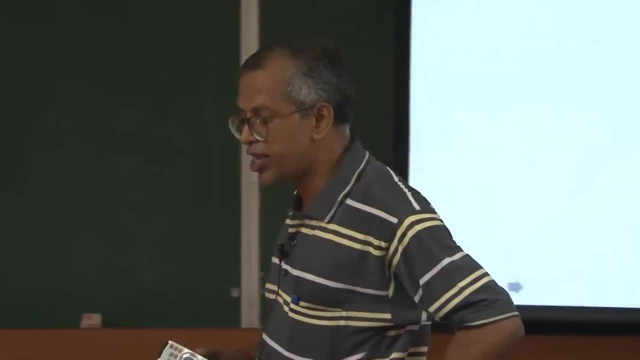 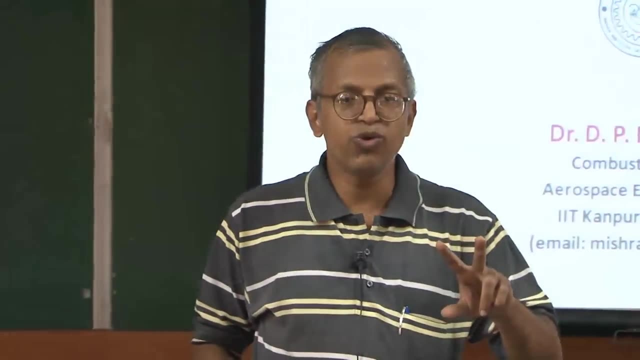 others. that is another mythological story I would like to share with you. that is about Greek mythology. There are two person. one is father Daedalus and his son Icarus. Who is the father of Icarus? Who is the father of Icarus? 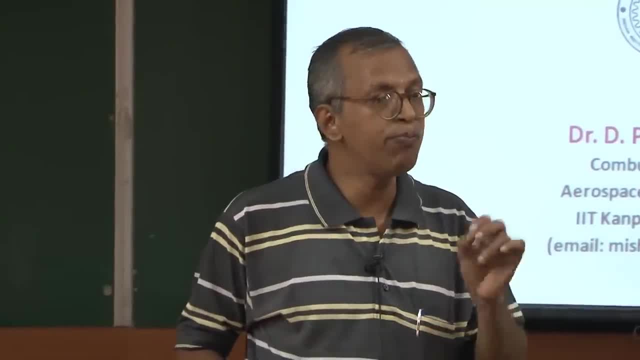 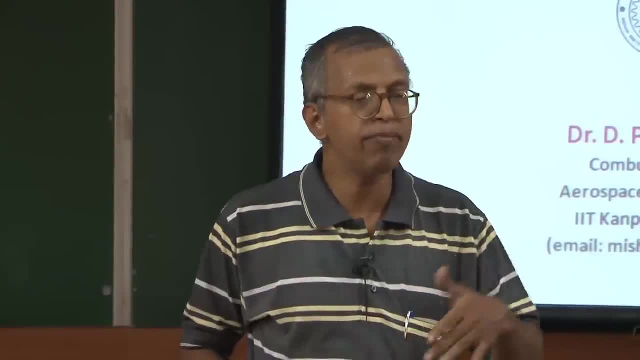 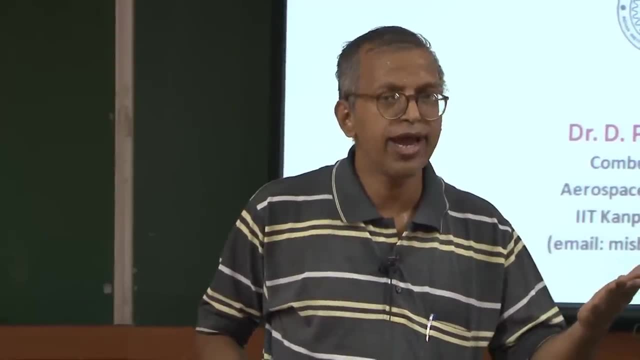 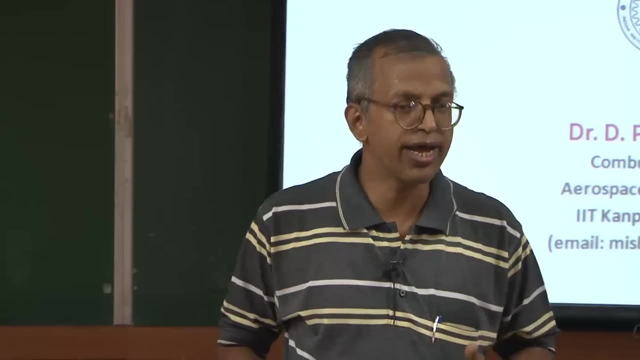 Munich and they try to escape from the jail, Made a conspiracy and by using the principle of the flying and they made the wing made out of wax and feathers. You know, like Icarus, who is a young and enthusiastic, he did not listen to the advice of his father. 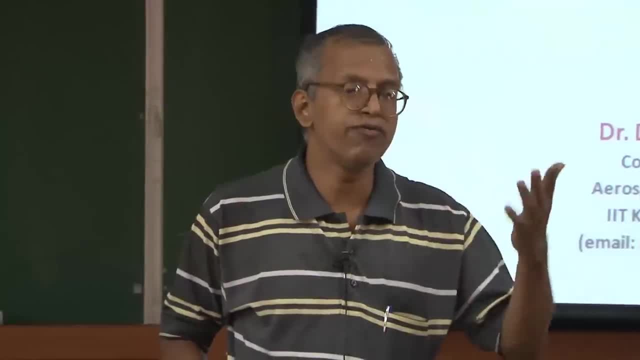 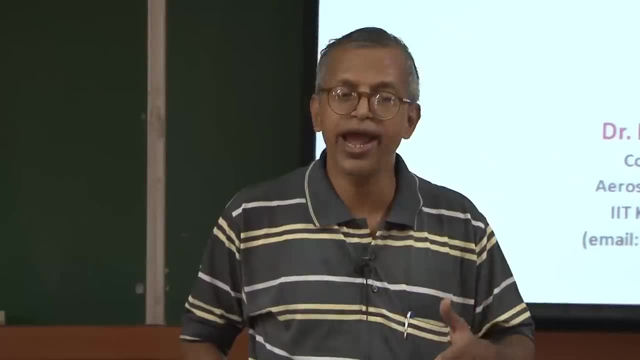 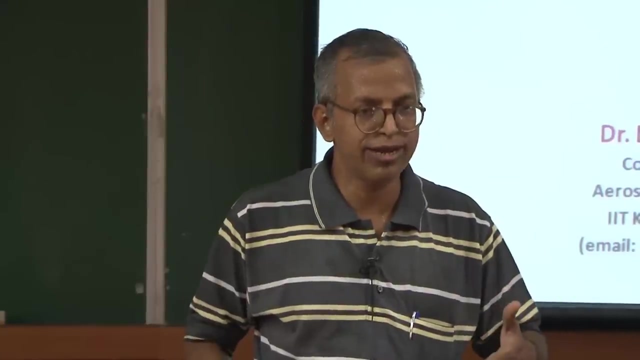 to get it out of his and he flied, of course, to a very high height and, because of sun, the waxes got melted and he dipped into the mediterranean seas. as a result, he was being caught and put into jail. So, if you look at, there are several attempts, several things have been told, stories are. 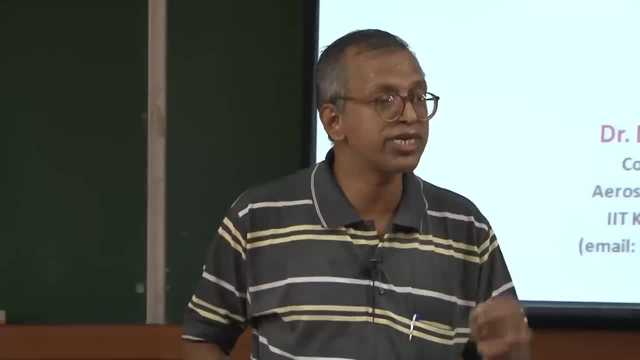 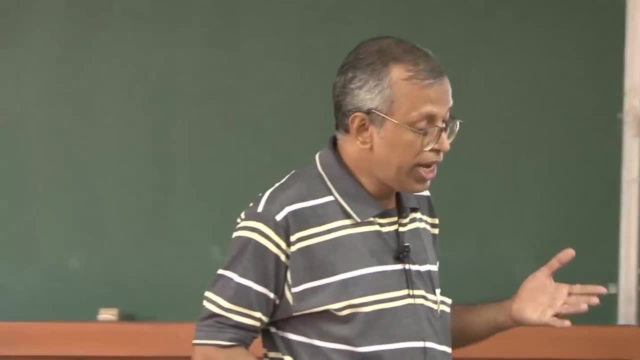 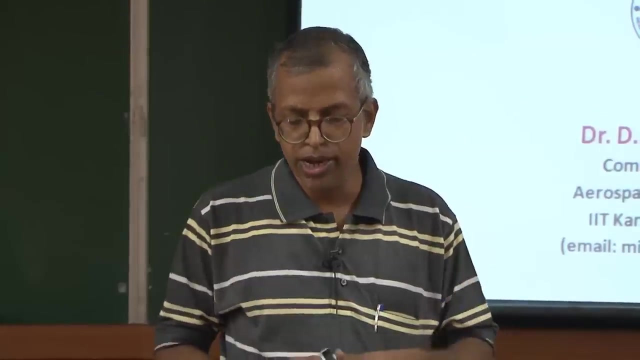 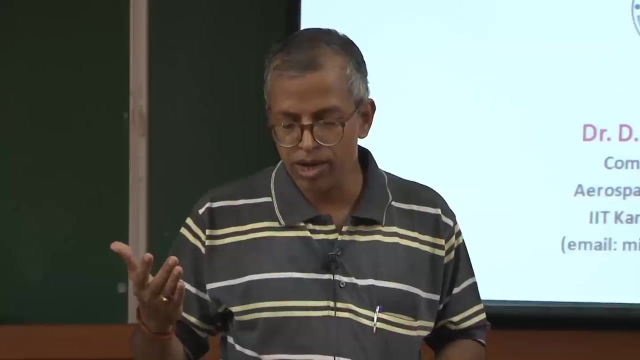 being floating around how many failures they have made. but still, people have tried. and later on there is a- what do you call the Sir William Calais, who was made a, basically a. what do you call mimic the flight of a kite? and made a. what do you call a glider right? 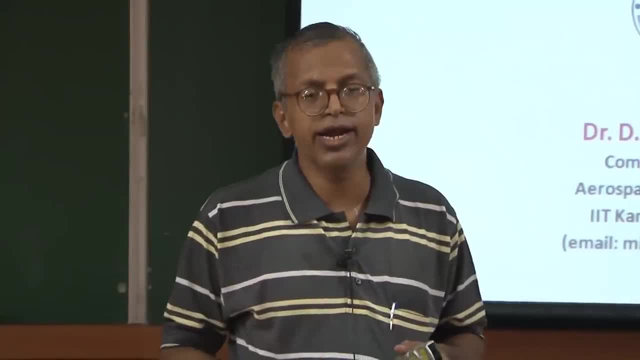 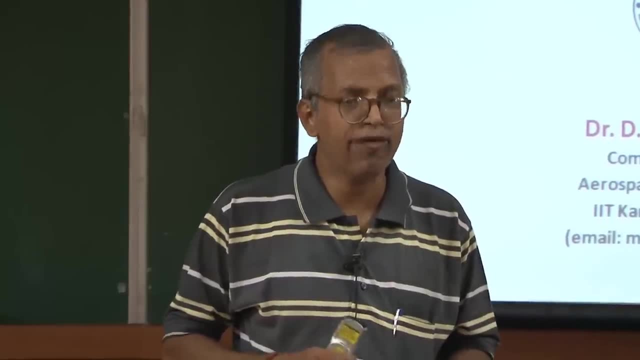 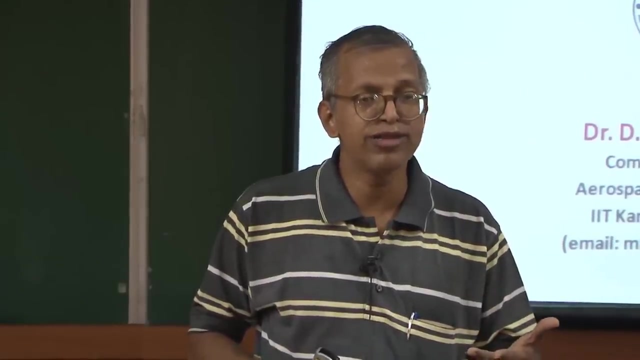 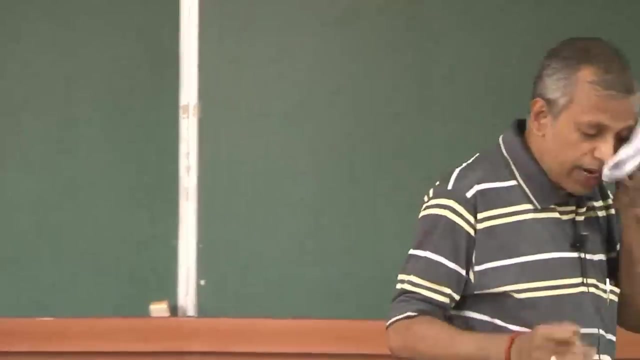 in 1804.. And after 100 years, there was a person known as Wright brothers Who made a epoch of flying an aircraft. we will be discussing more about Wright brothers achievements and there starts the era of the aerospace propulsion. you might be knowing the story of Wright brothers and other things. Now let us ask a question: what do you mean? 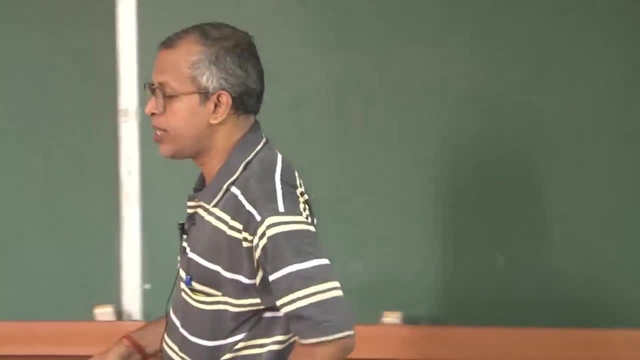 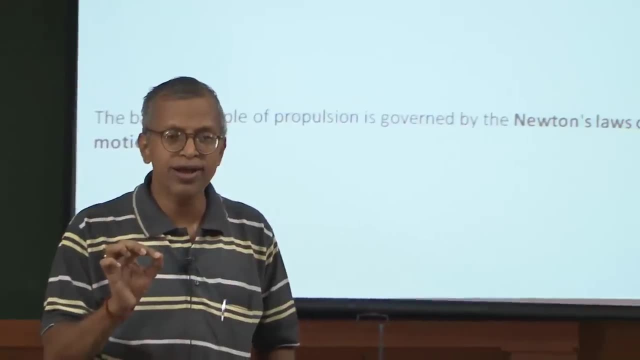 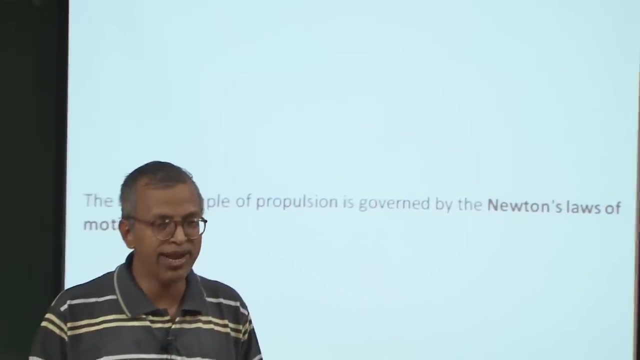 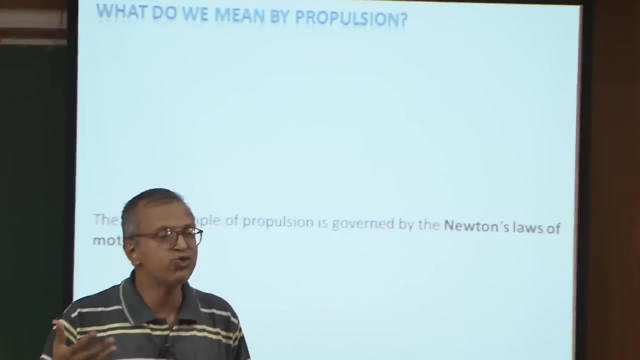 by propulsion. can anybody tell me, like what do you mean by propulsion? Propulsion is basically stands from a word Propulsion, known as propel. it is basically a verb. what it means. it means to propel right. to propel means to make or cause a motion to an object or a body, And when we are trying 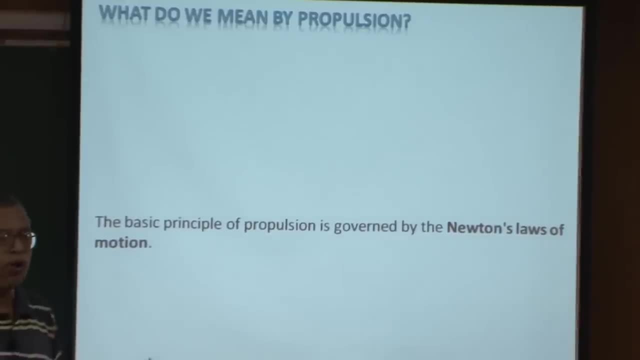 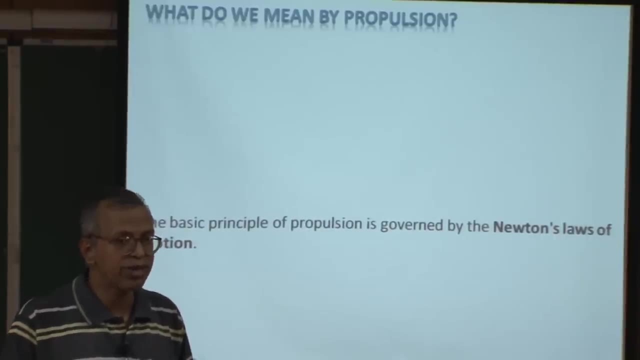 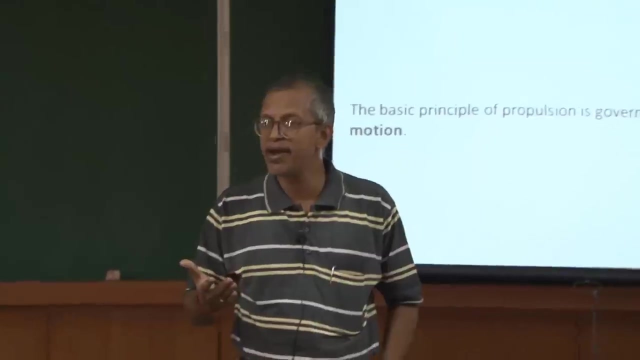 to impart a motion to a body or object. what we need to do? we will have to apply a force. Is it possible that we can apply a force in start moving? certainly no. it will be unbalanced force, such that it will be overcoming the inertia, right or a resistance, And it must. 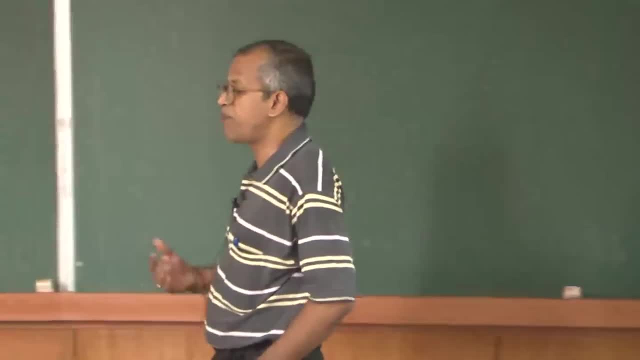 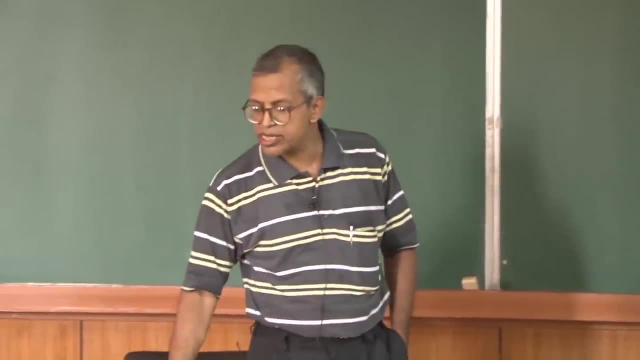 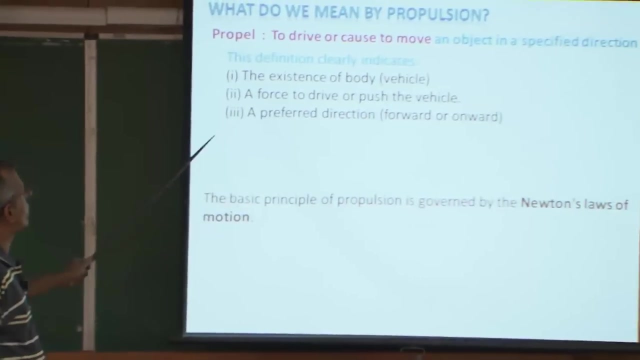 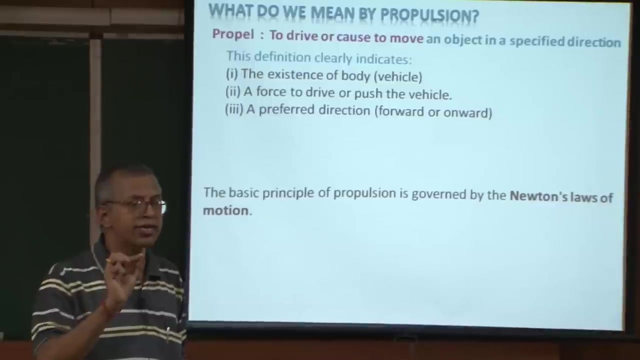 be in a specified direction. specified direction means for a particular direction, whether it will be forward or a backward or a side wise, This definition clearly indicates the existence of a body And a force to drive or a push a vehicle, and this motion will be in a preferred direction. that is a, for example. if I look 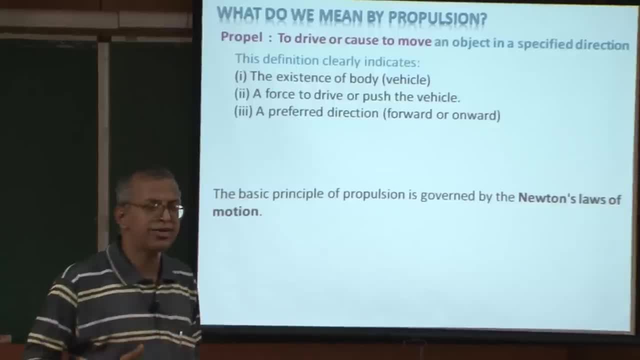 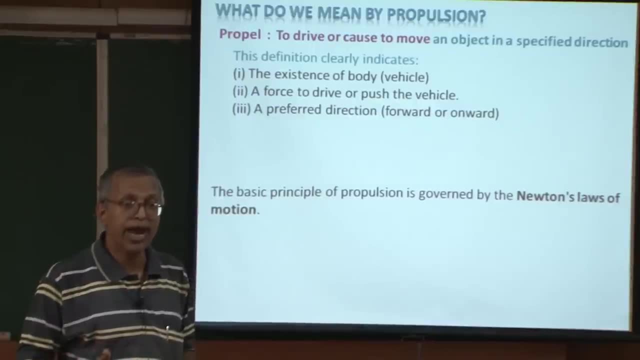 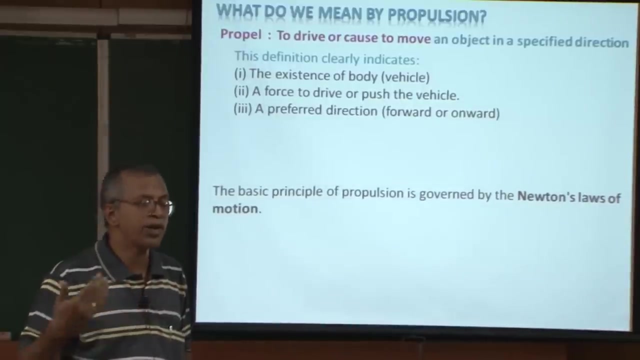 at I walk, is it in a preferred direction? how I am walking, is it I am applying a force or not? And in applying force, how it is acting on the body. So these questions, all of you will be knowing, but we will be discussing in just to make. 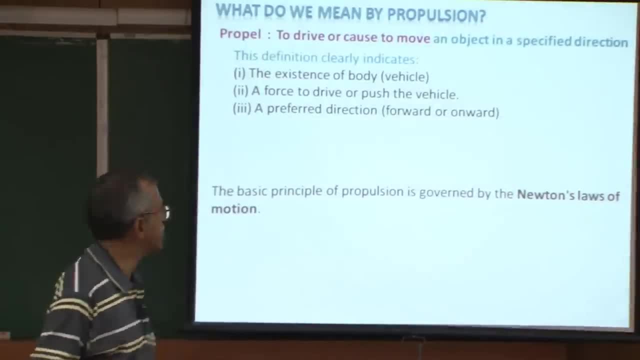 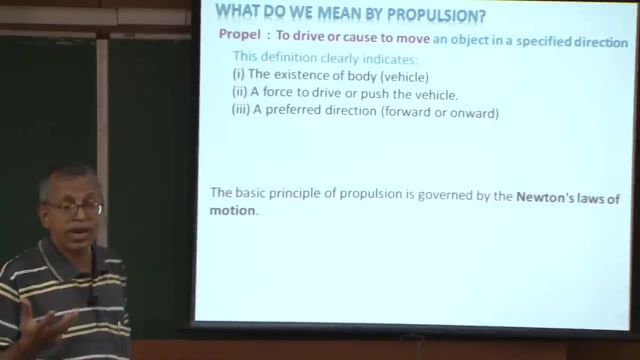 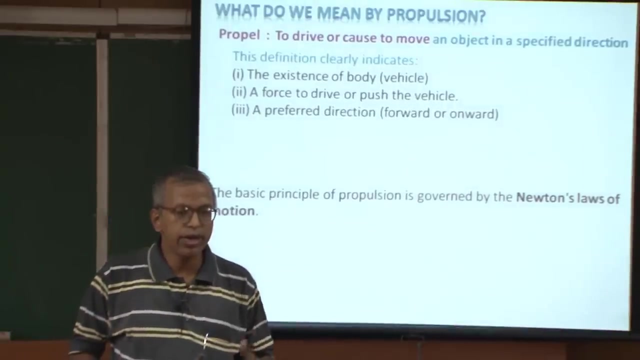 in more clear and have a feel for it. So if you look at, these are basic principles or what you call. we mean propulsion. Now when you talk about propulsion, suppose the insect is moving, or a what you call a snake is moving on the grass or a ground or a fish. 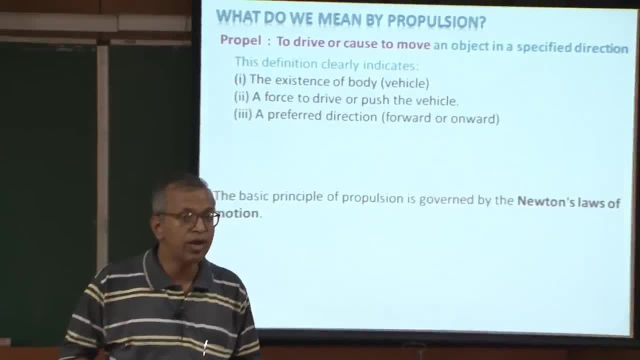 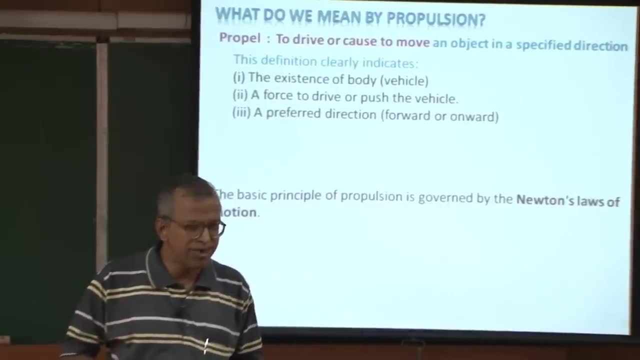 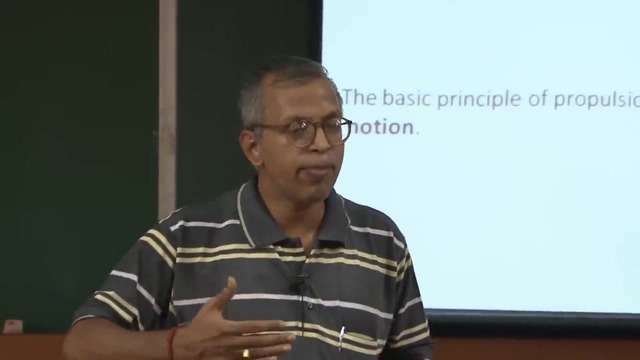 is moving in the water. will you call it as a propulsion or will you call it something else? Naturally, propulsion, but we never use those term whenever it is moving. very often, However, because it is related to the motion. it is related to applying a force which will 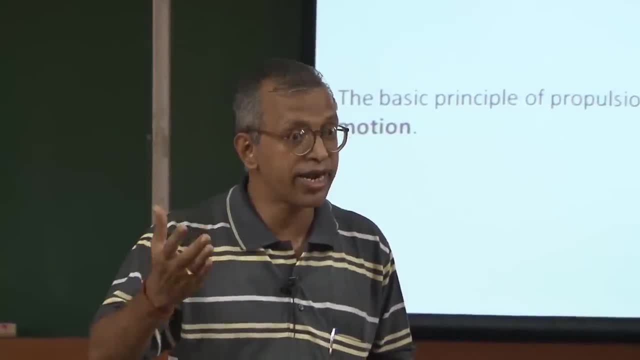 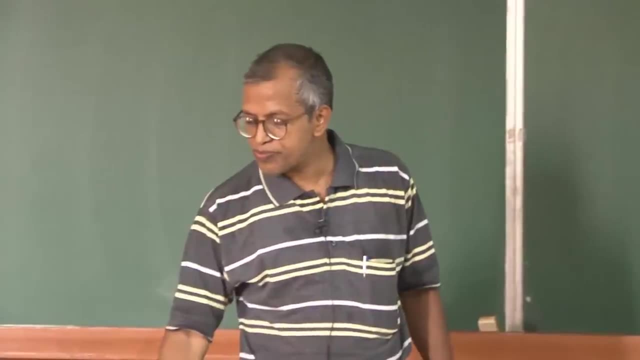 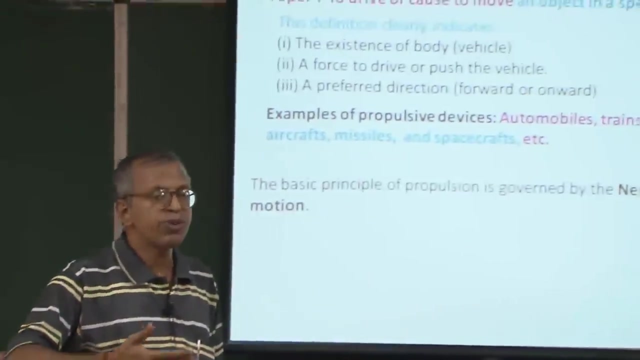 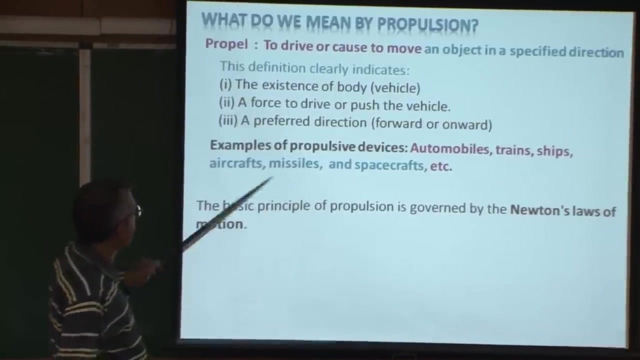 make it the motion in a particular direction, So therefore we call it as a propulsion. However, there are several devices which Are like automobiles, trains and ships which are being to be propelled, and for that we need to have engines. Similarly, we will be looking at in this aerospace propulsion that 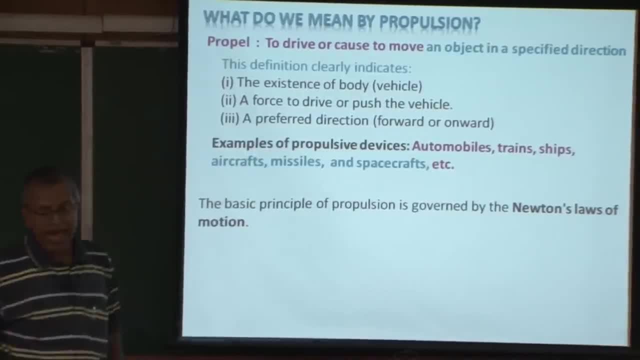 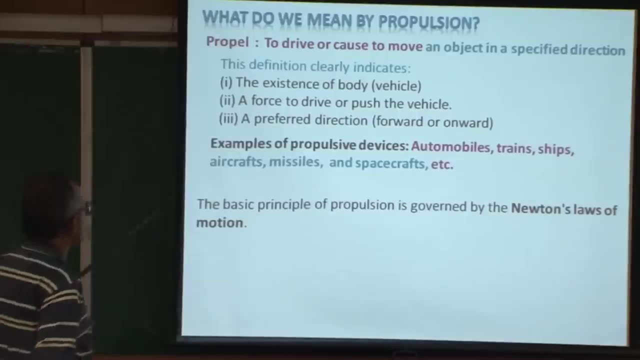 propulsive devices are aircraft, missiles and space craft and several others one can think of, but we will be concentrating on this. Then question arises: what is the propulsion, What is the basic principle which will be governing the propulsion process? So we know. 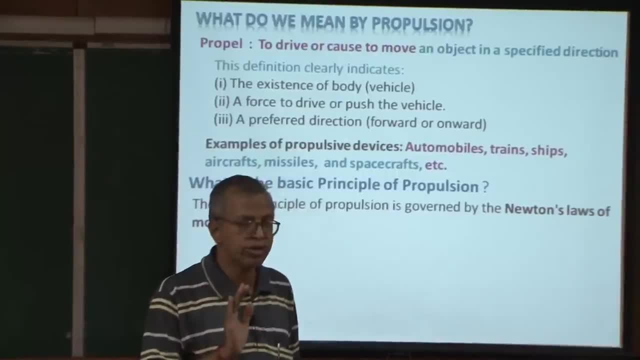 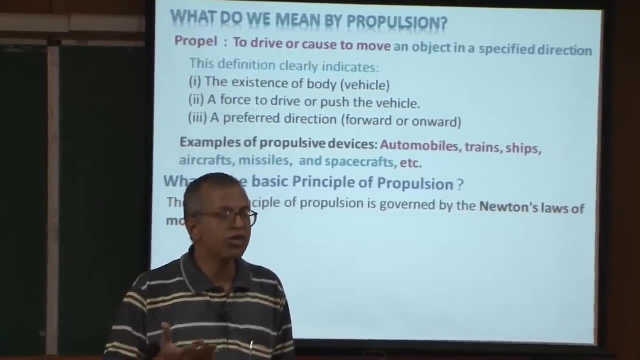 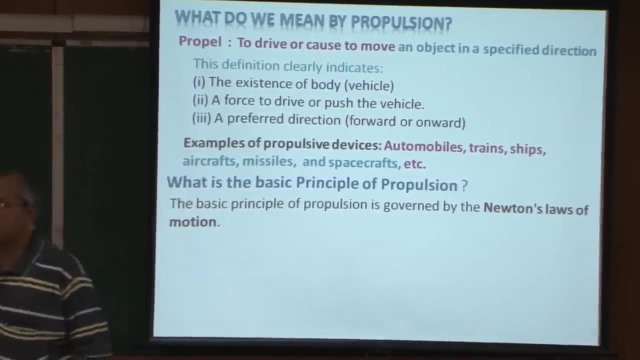 that one has to apply a force and it will cause an motion. Now, whenever it will cause an motion, then naturally laws of motion comes into picture. You must have studied all these things in high school. violator, You have a feel for it. What is this? laws? If I say, what is first law, what is second? 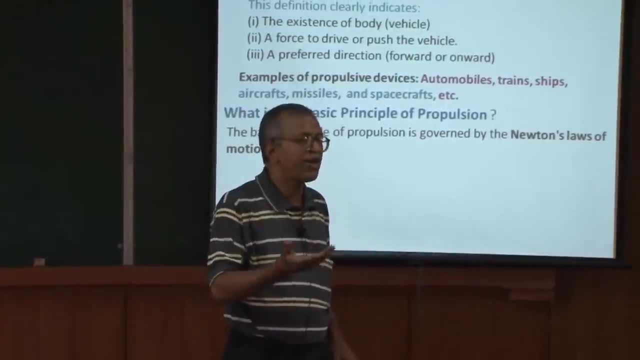 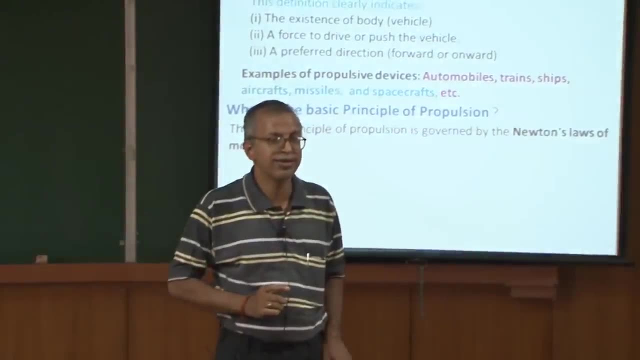 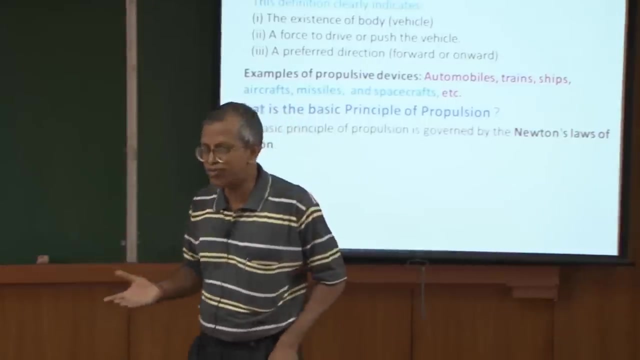 law of motion and third law of motion. Some of you may tell me what it is in words, But did you experience those things? That is more important to have a experienced than mugging it up or remembering certain laws or applying it in mathematical sense. I will take an example. 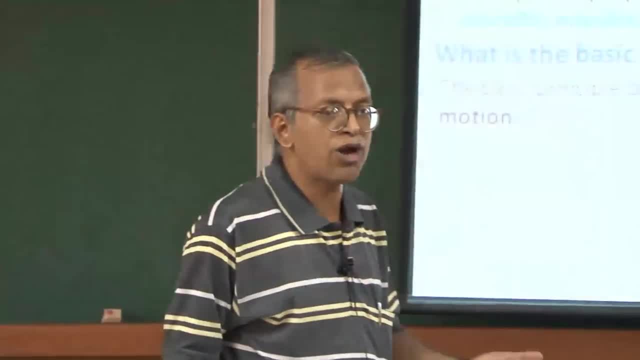 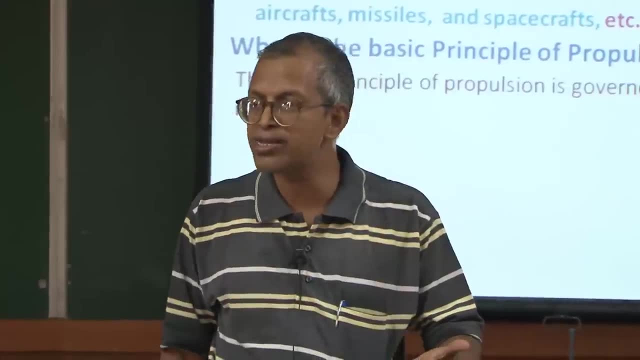 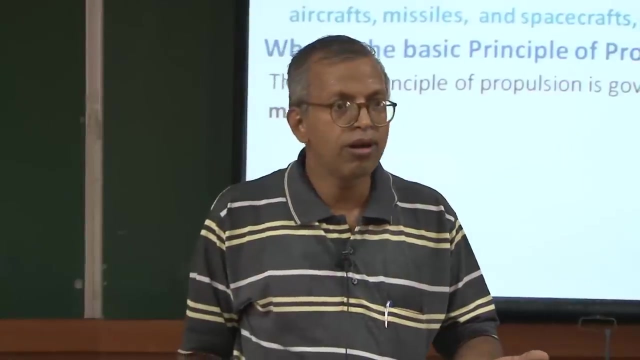 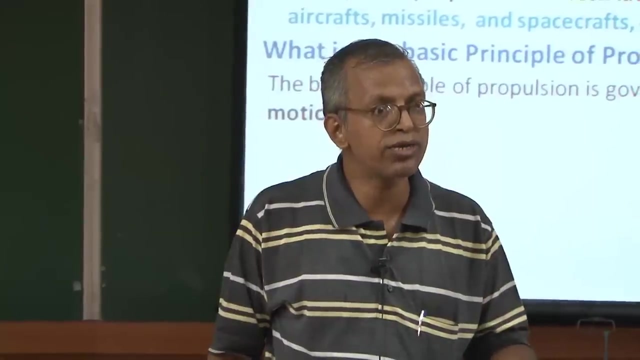 a child experience these laws or not? If you look at a child may be two years or one and a half years child. will it be experience these laws of motion or not? But you know if they are experiencing but whereas when we grow up we are not experience. I will give an example. 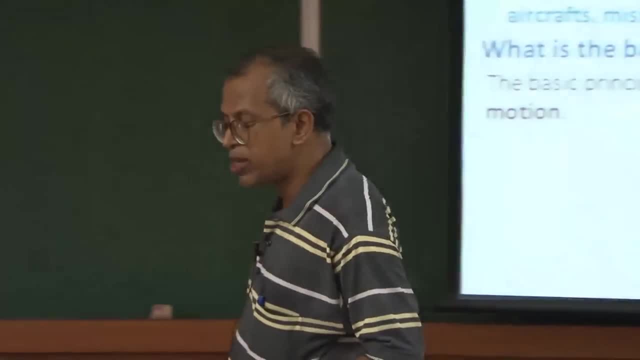 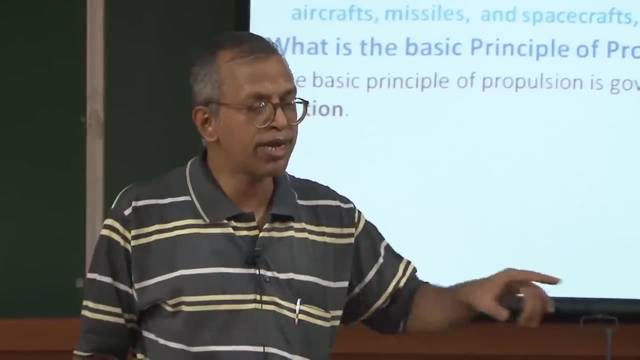 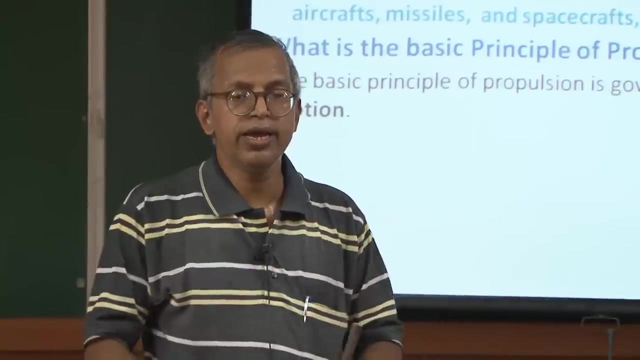 how they are experiencing. and you might have observed a child has kept a toy in one place. you will move around and come and see whether the toy is lying there or not. in the same, exactly same place, Let us say a baby or a child is playing with a car toy and you will. 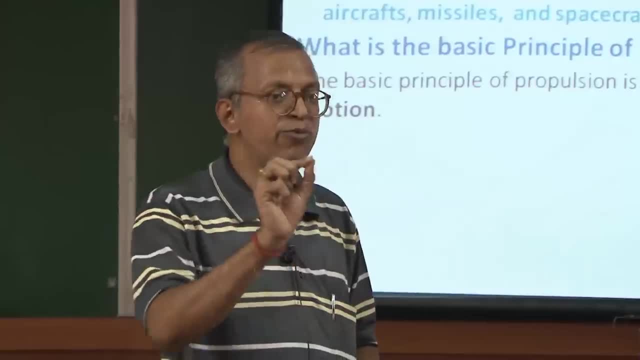 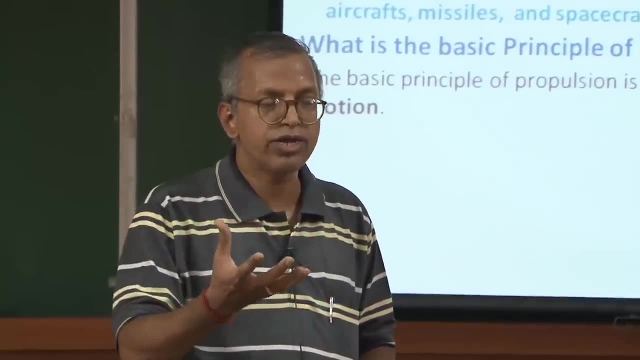 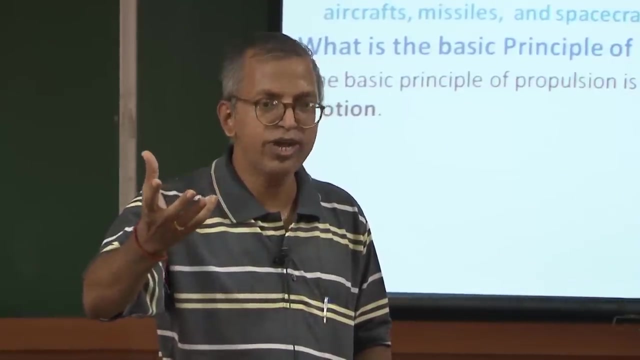 push the car in a particular direction such that it will move and reach and you are going and catching a, let us say, ball. you know lot of children like to play with the ball. Like you will be throwing to a ball to another person, another child will catch it, or sometimes 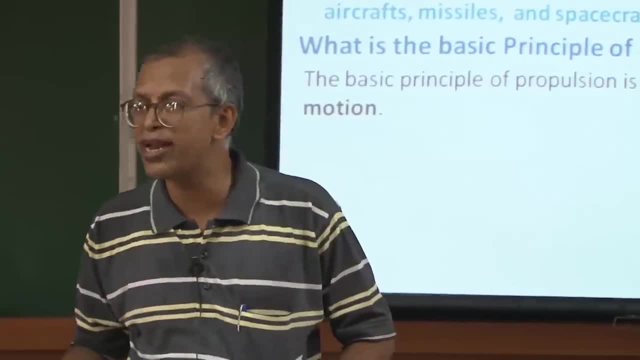 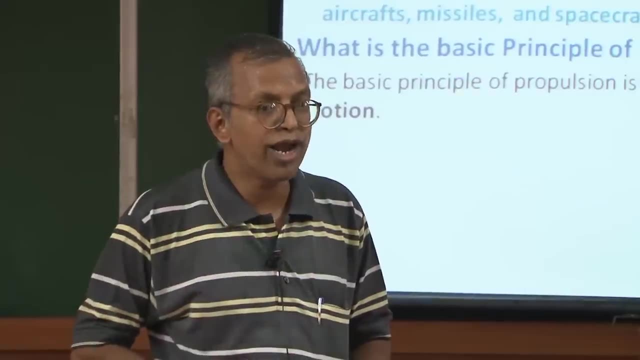 the, you know, single child is not having way to play or interact nowadays it is the go of the world. So they will be put what you call throwing the ball towards the wall and rebound it back and they catch it. So what it indicates 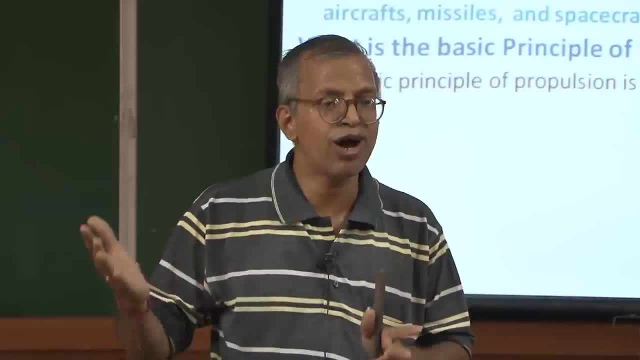 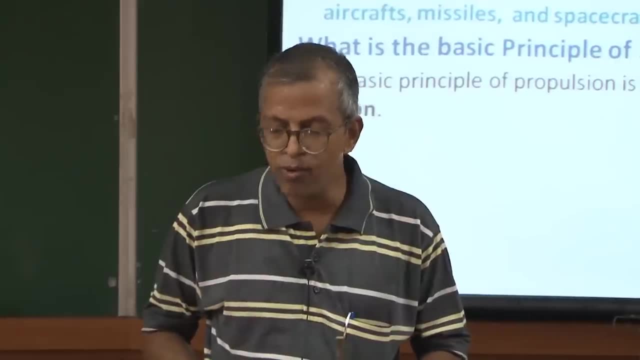 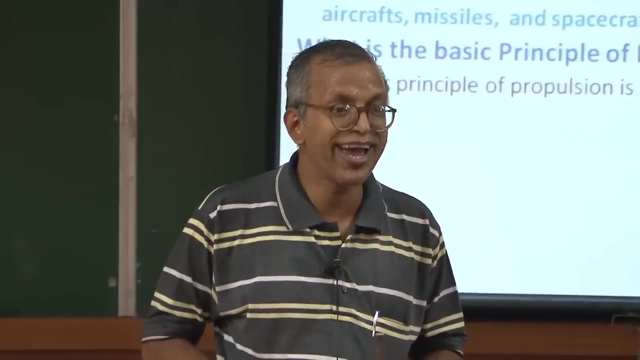 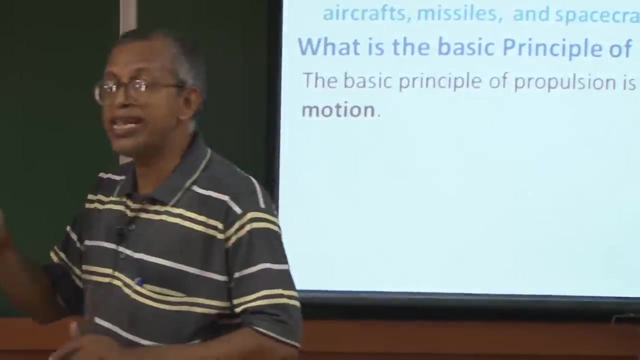 That is, they are experiencing all the three laws of motion. What are those? first law of motion? Can anybody tell me like? what is the first law of motion? Now, please tell me. in a words, inertia is right. That means a body will remain in the state of rest or of in uniform. 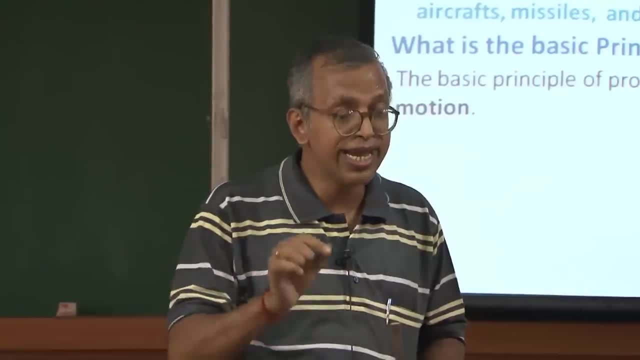 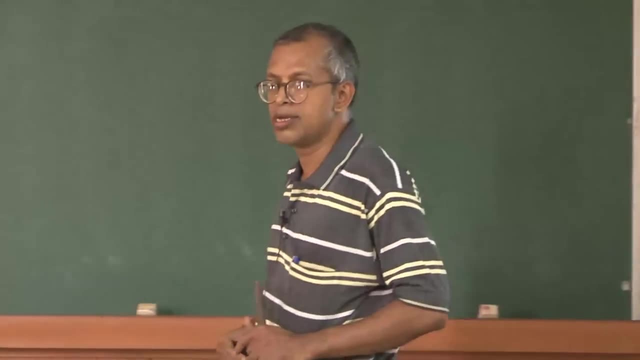 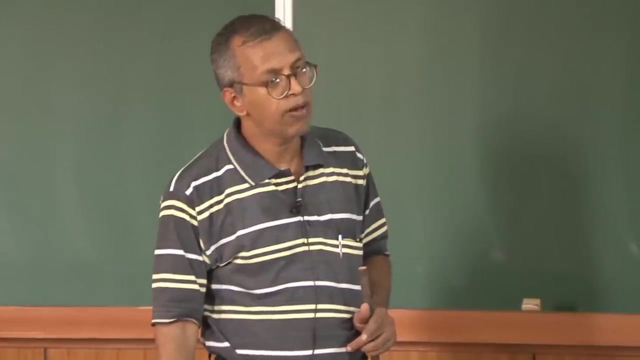 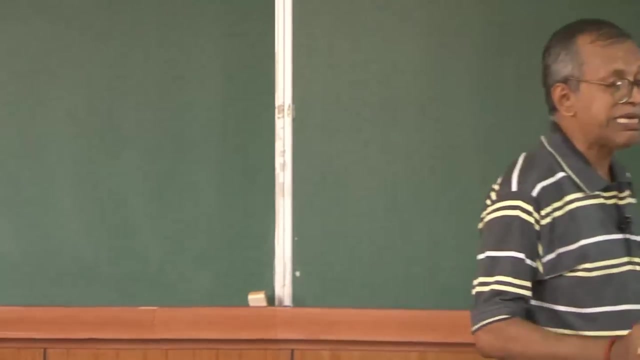 motion Along a straight line, unless it is acted upon by an unbalance force. What is that unbalance force? That means, if it is there, I will apply a force. will it moving? It is not moving. I am applying a force. but if I will apply more force, then it is moving. That means a force. 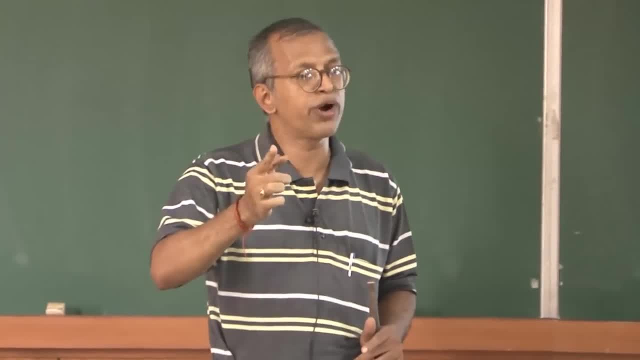 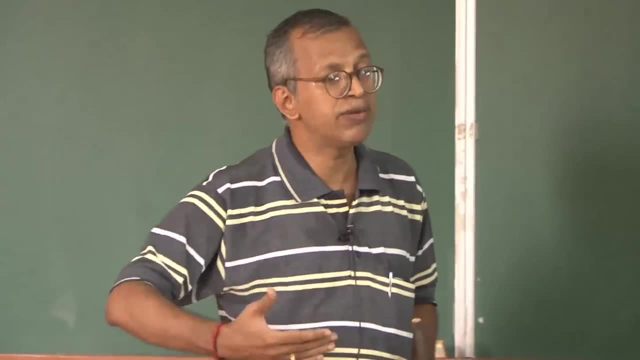 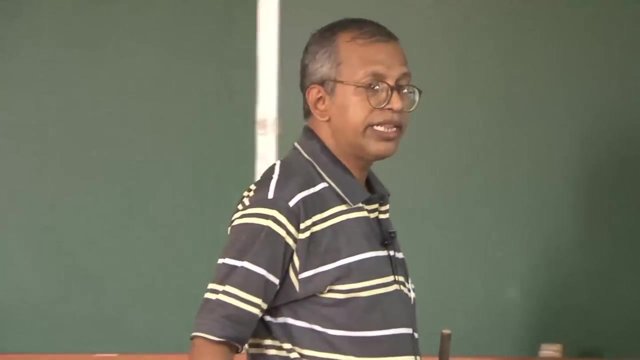 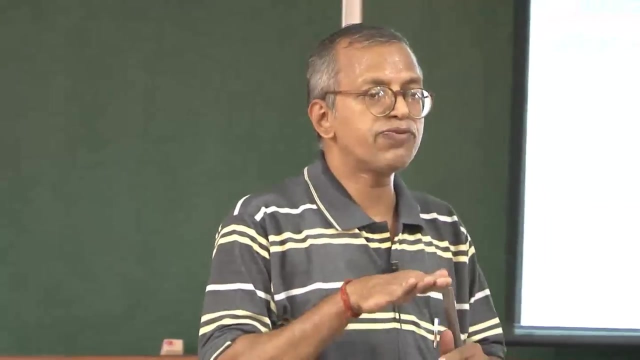 which is acting is unbalance force that will make a body to move. Now, how will relate this unbalance force to the change in the motion? something is changing in the motion, right, and in this case there is a friction which is occurring. there is a friction. So whenever friction is there, this force, whatever I am applying, must overcome. 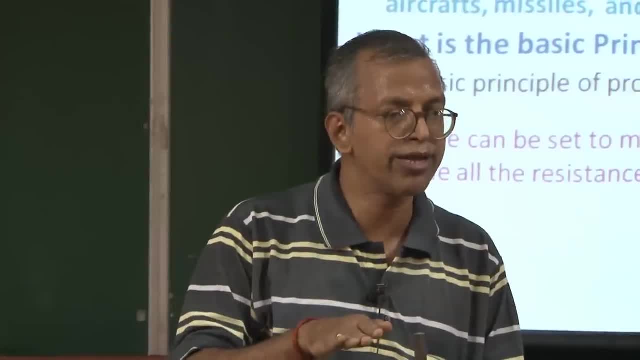 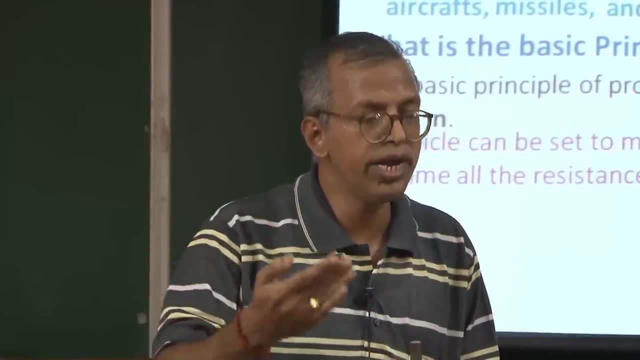 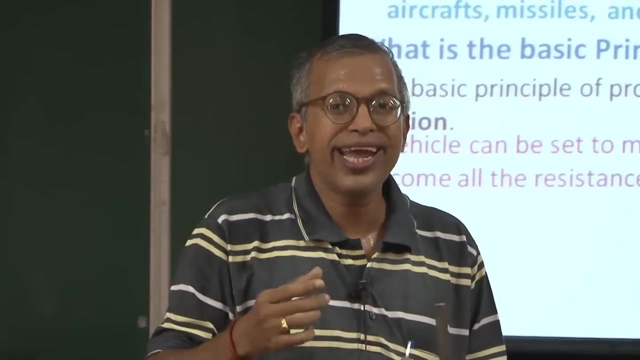 the frictional forces between the surface and the body right Now, then only it will move motion. it will make a move or it will be in motion, or motion is imparted to the body. Now, if you look at like what really changing whenever an unbalance 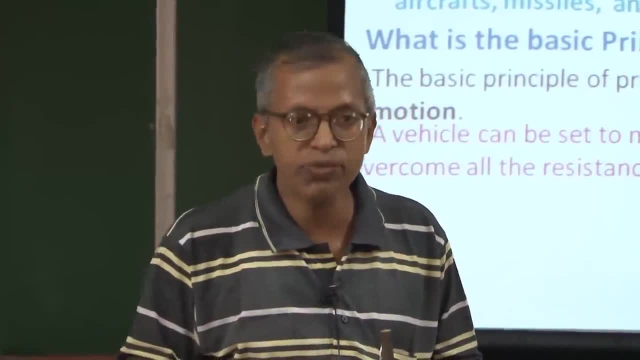 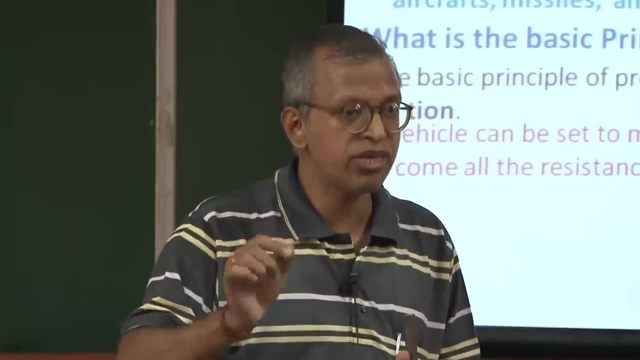 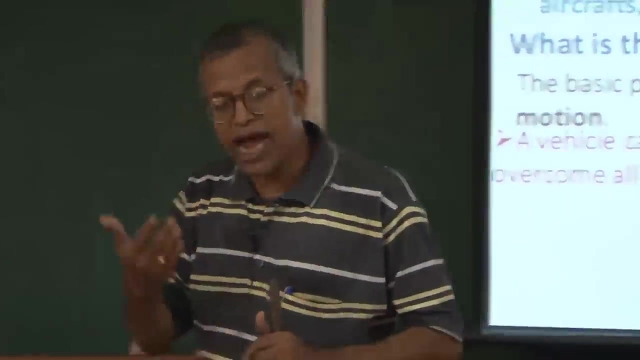 force being acted upon a body. What is being changed? There will be change in moment. that means rate of change of momentum will be proportional to force. So therefore, in that case that we call it as a second law of motion and this momentum, 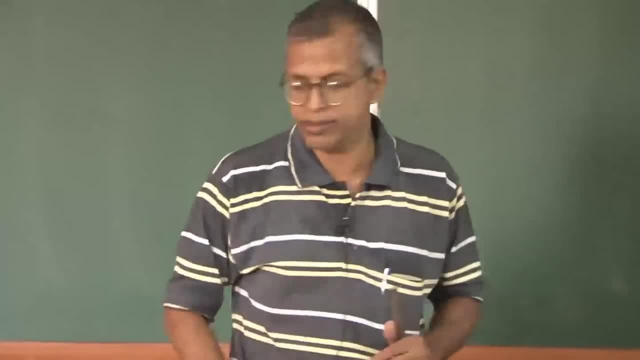 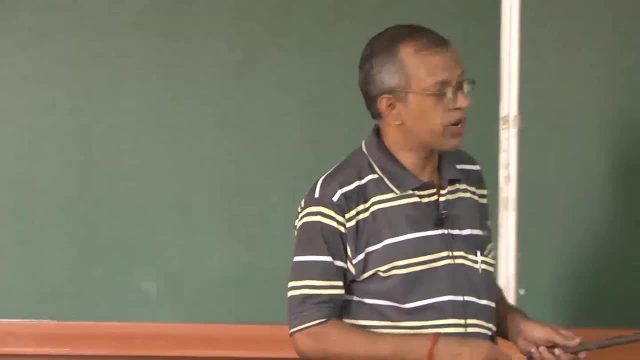 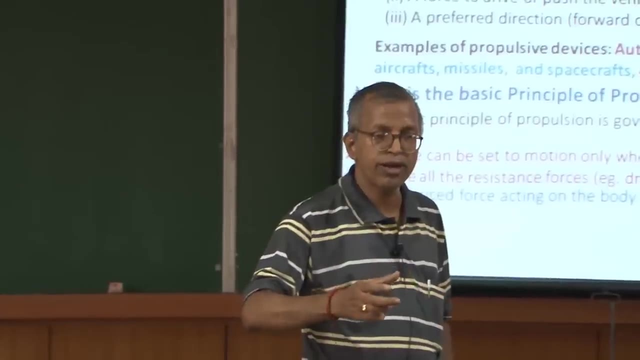 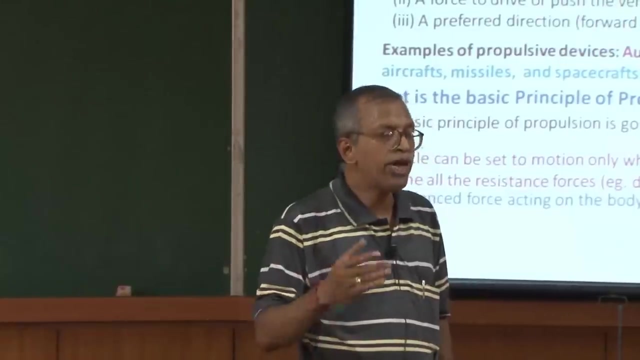 will be in the direction of the applied force or the unbalance force, right. So unbalance force acting on the body produces an acceleration because there is a change in the momentum of the body. mass can be changing, or so also velocity, Or both of them will be changing. but when we will consider the mass to be constant, then 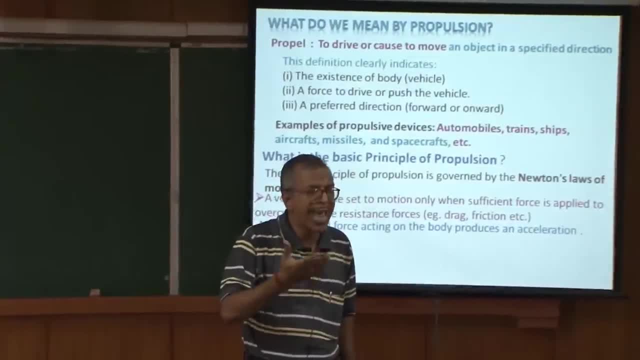 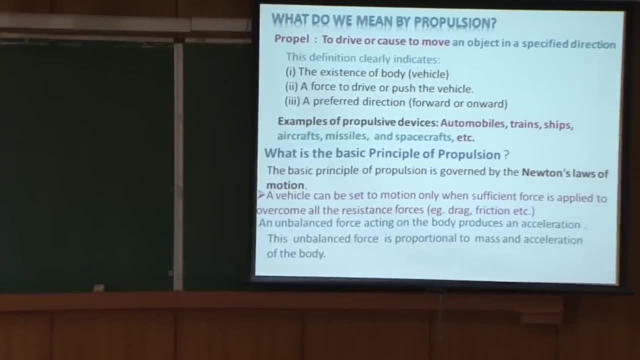 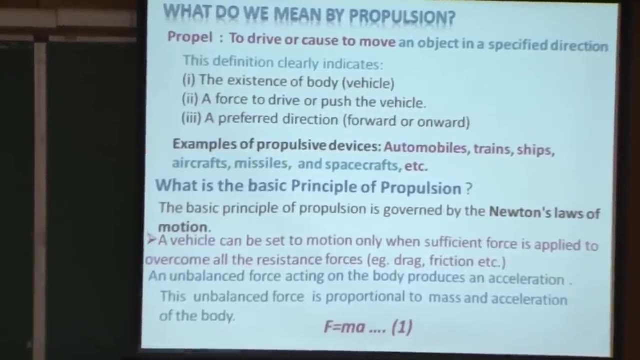 change in velocity with respect to time. we call it as a acceleration right. So therefore, generally, we consider the second law of motion, in which unbalance force is proportional to mass and acceleration of body is known. as it can be expressed is a mathematical formula. 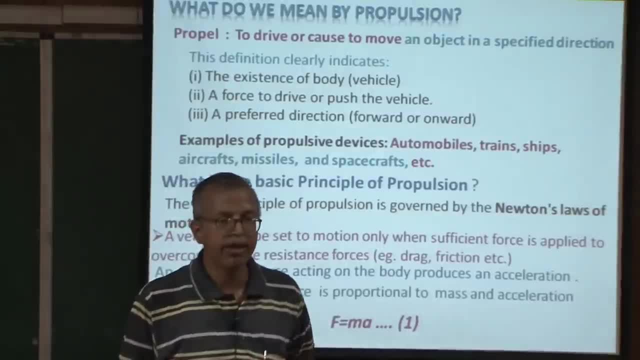 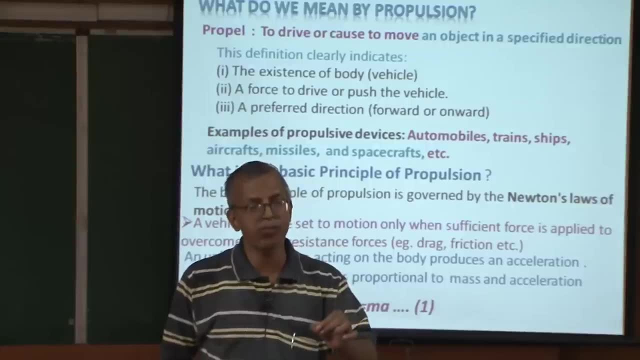 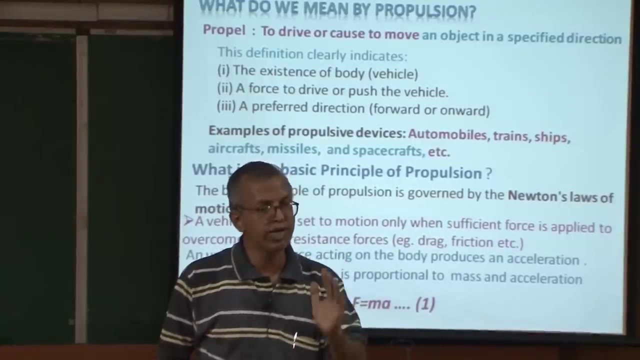 which all of you know. So, therefore, this is the law of second law of motion. then what is the third law of motion? 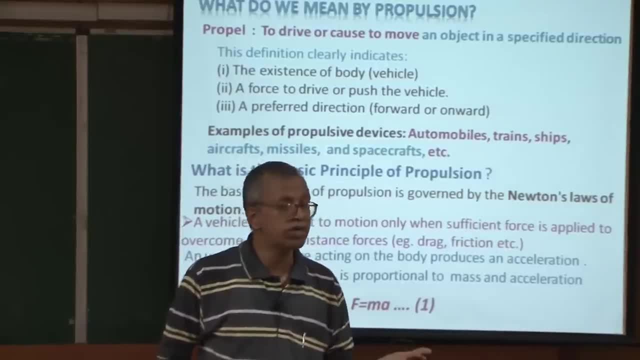 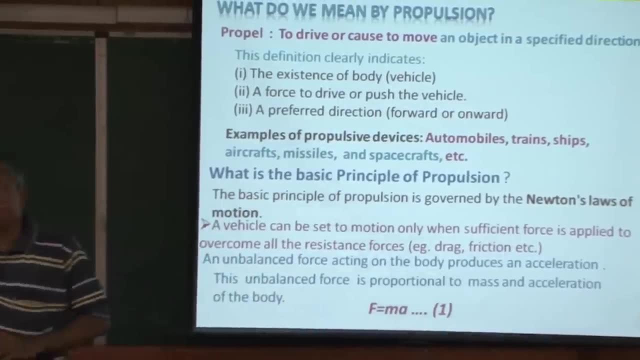 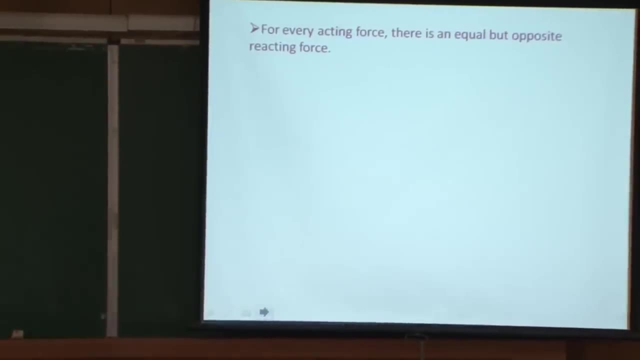 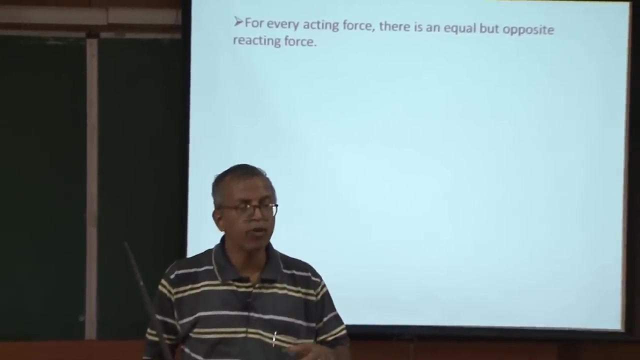 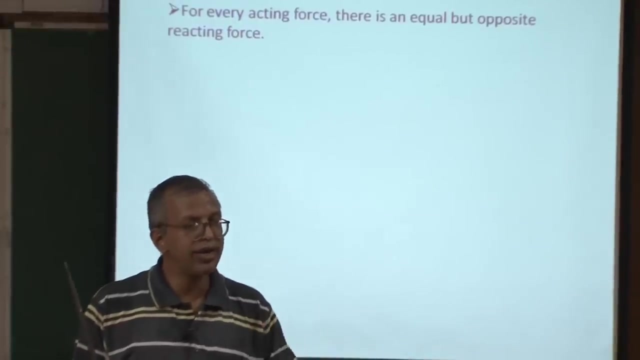 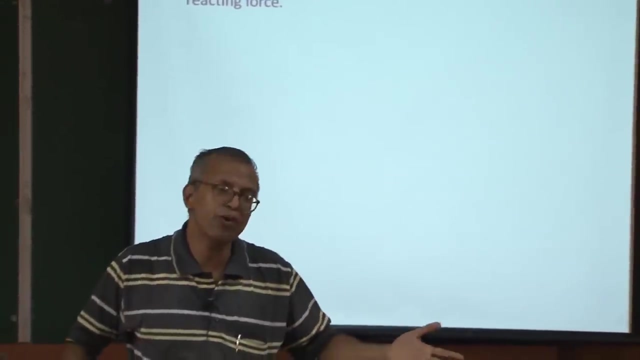 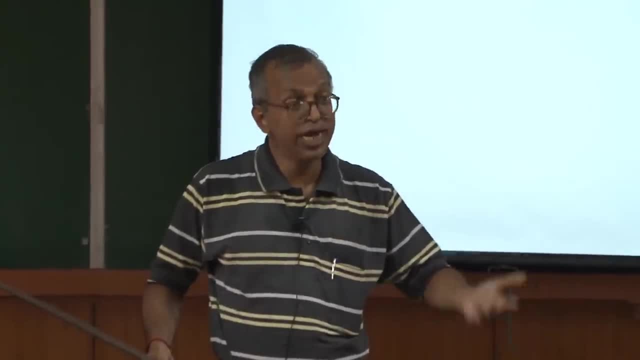 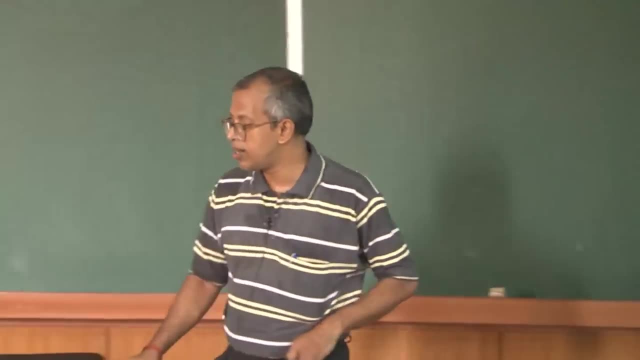 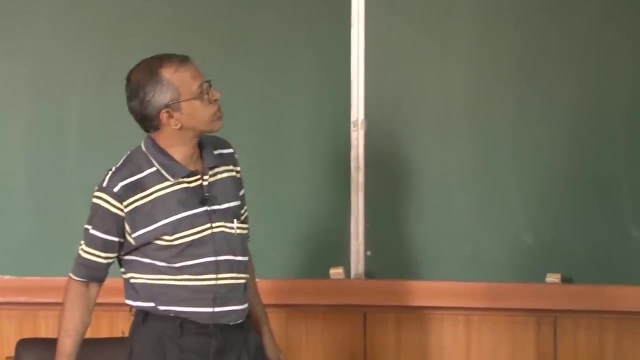 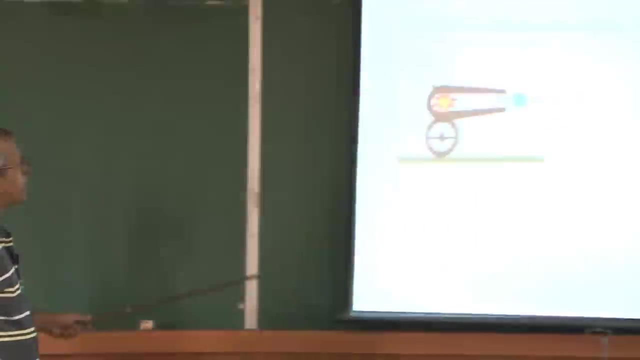 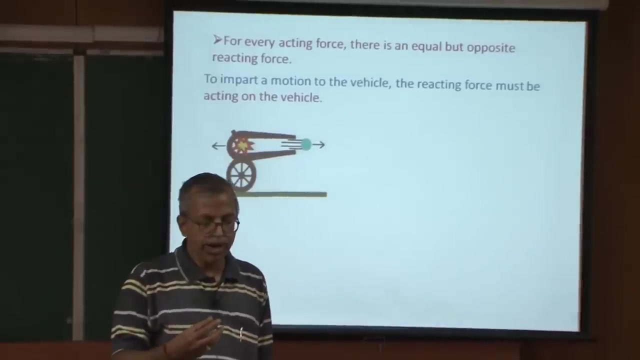 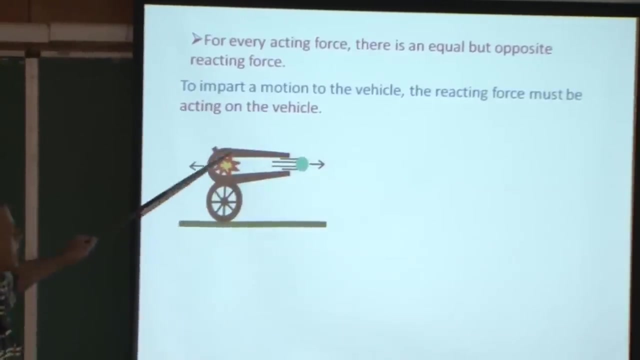 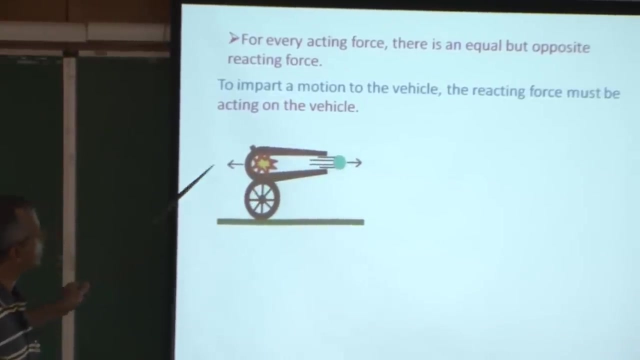 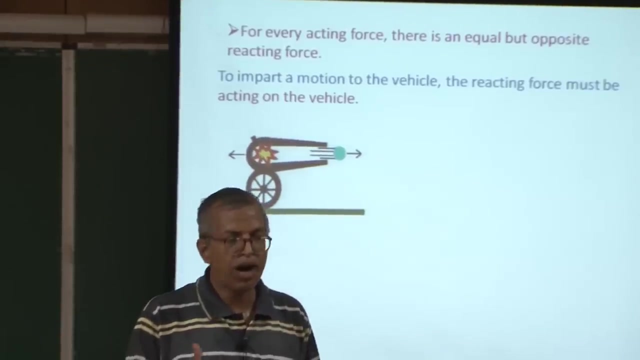 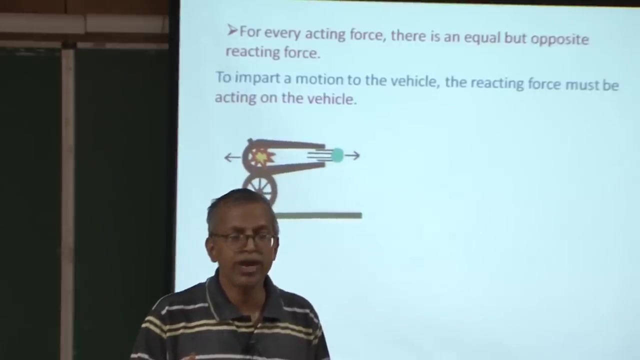 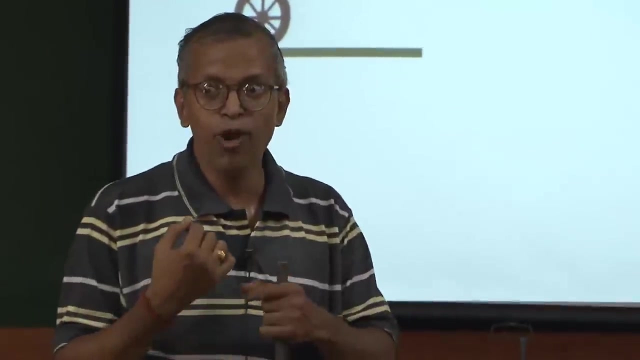 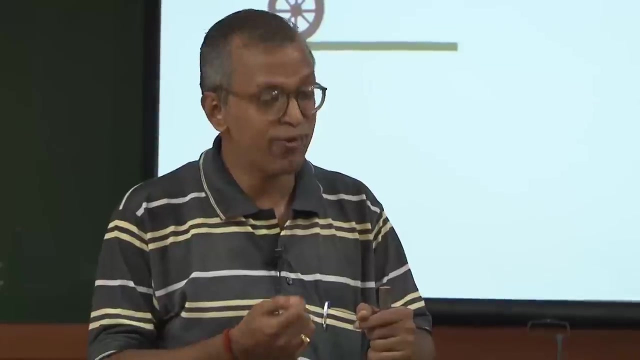 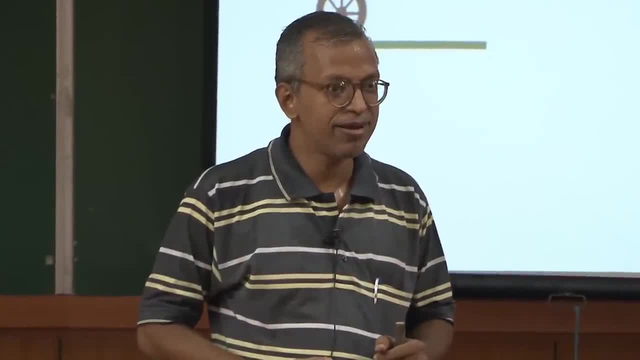 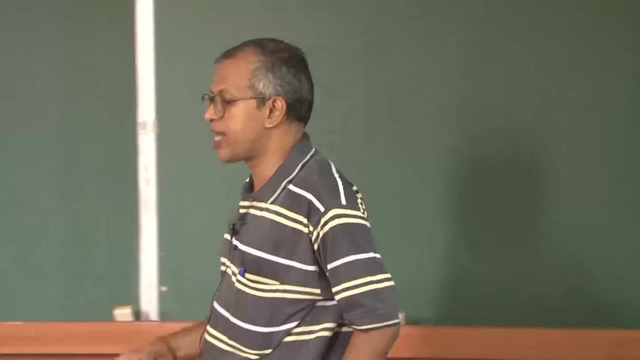 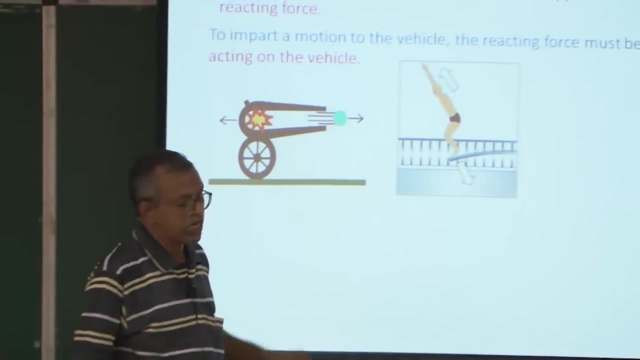 it came and hit my body because it is moving, So opposite reaction is there. Similarly, several other things one can think of. for example, like there is in the swimming pool, there will be a spring board on which you will try to push and then you will be jumped. 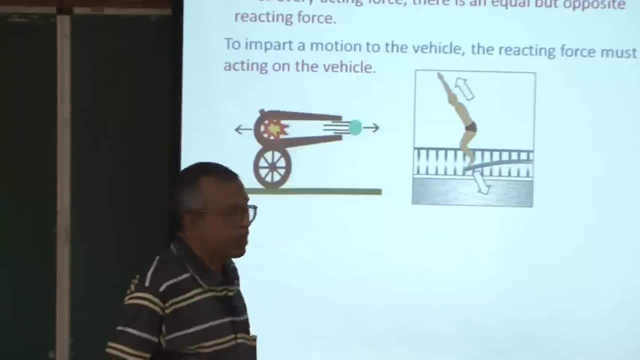 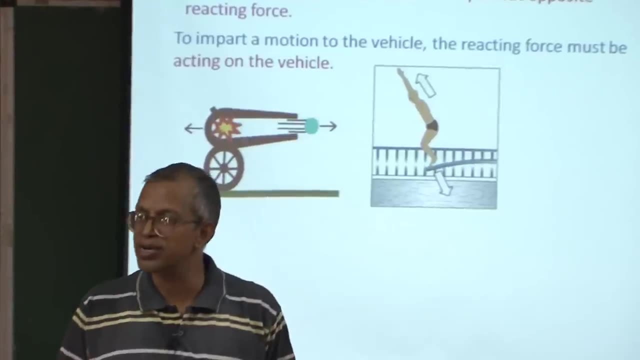 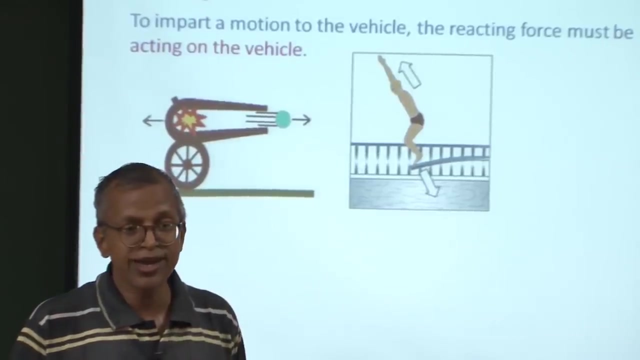 and put into the swimming, what you call swimming pool. So this is a another example. the way we walk is also by the third law of motion, And in our scriptures we talk about every action as a equal but opposite reaction. that is known as law of mass law, of what you call. 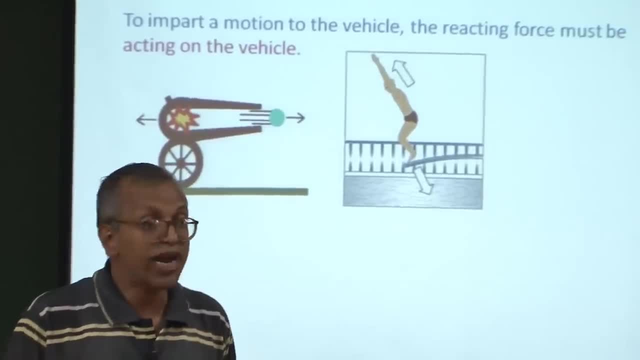 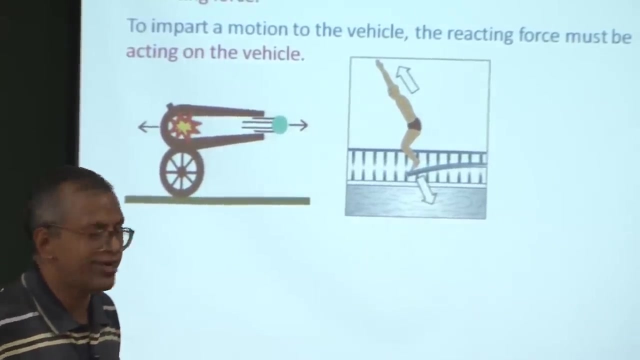 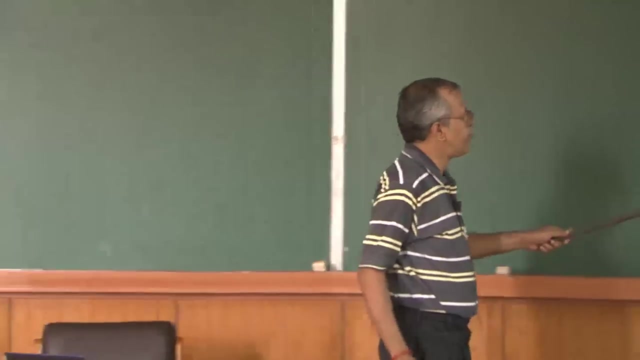 karma, So that some of you may not be knowing what is that nowadays people are not worried about, but it is very important to look at that law of karma, Which is similar to the law third law of motion, and so we will take a balloon, which 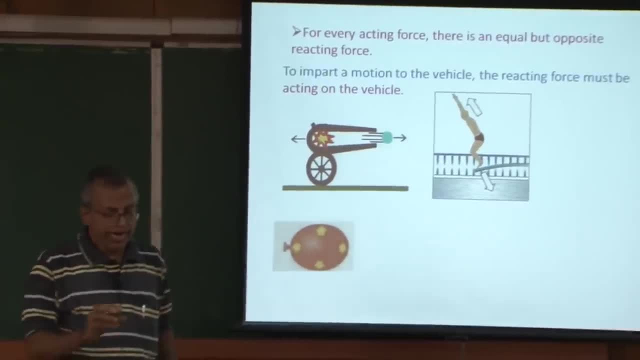 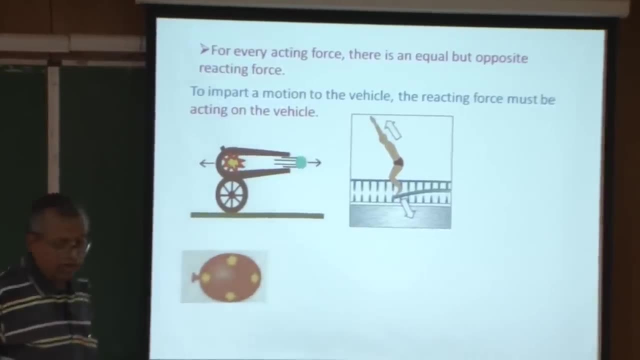 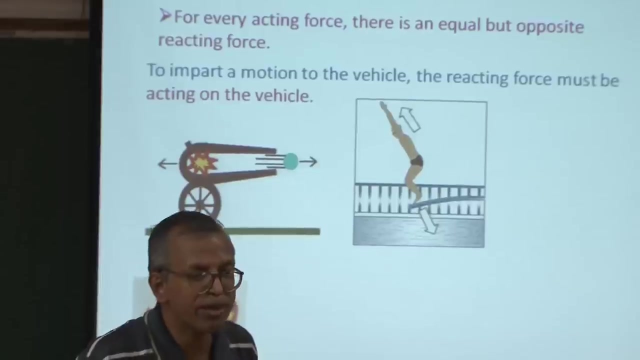 is in inflated one and it is in equilibrium because the pressure which is acting on this balloon, which is in equilibrium with the atmosphere, But however it is having higher pressure, you may think how it is It is happening because it is the elastic medium. So whenever it is in equilibrium, 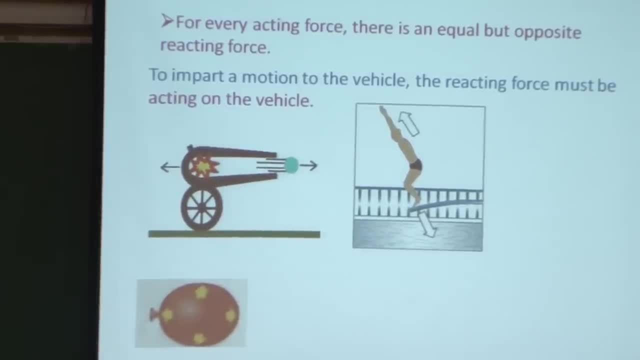 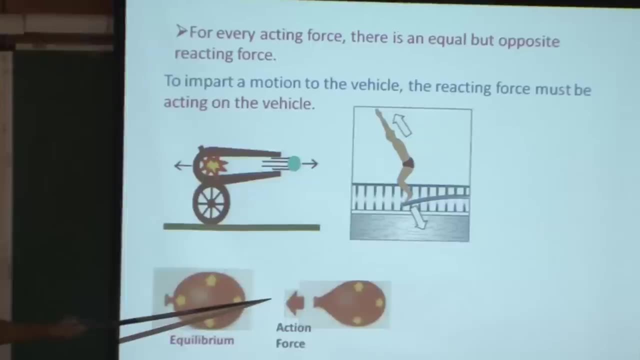 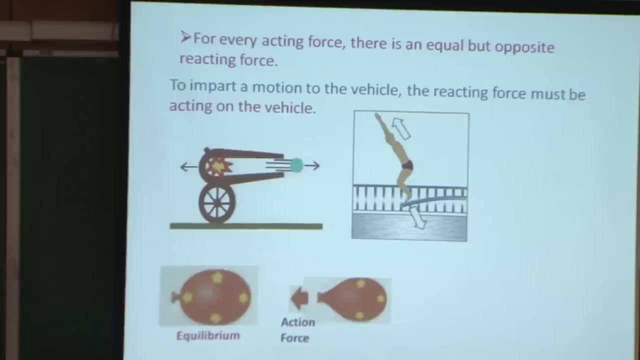 and if I remove this stem, allow the air to move, what will happen? The air will be moving out of this balloon and there will be an acting force, action, acting force or the action force- and there will be a reacting force along with this direction. As a result, the balloon will 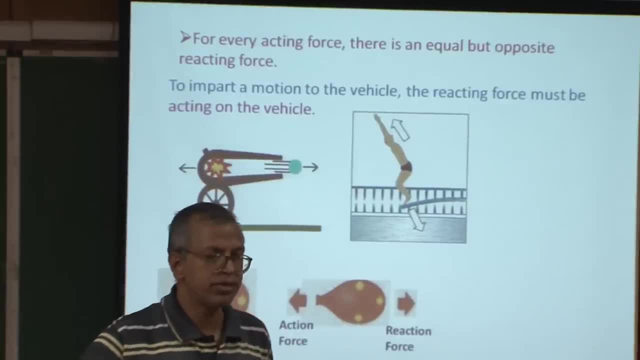 move away from the same place. This is a typical experiment, what people do, at least it is there in the high school book. but nobody does experiment today, either in the high school or in the secondary school, or even in engineering college. that is the fate of the our education system. 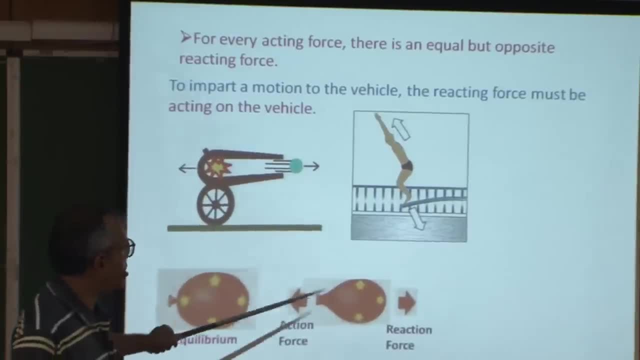 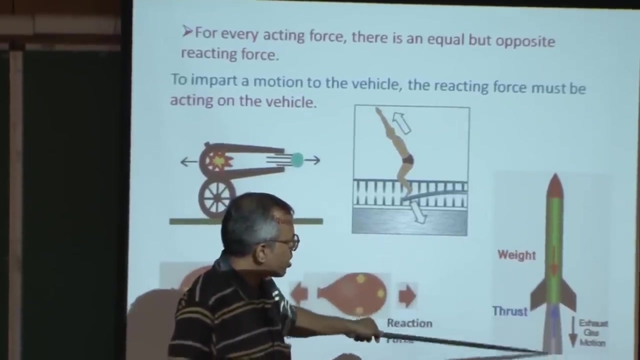 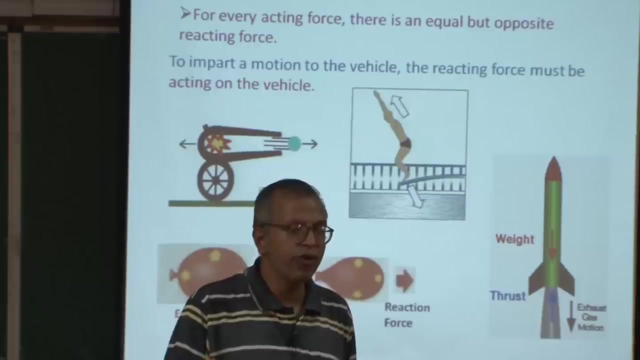 which is very bad. Now, if you look at, this is the basic principle by which the rocket engines you know being worked. So I will show you a figure where the hot gases will be ejected out of the nozzle. As a result, it will impart a thrust, and which will be- must be- much higher than the weight. 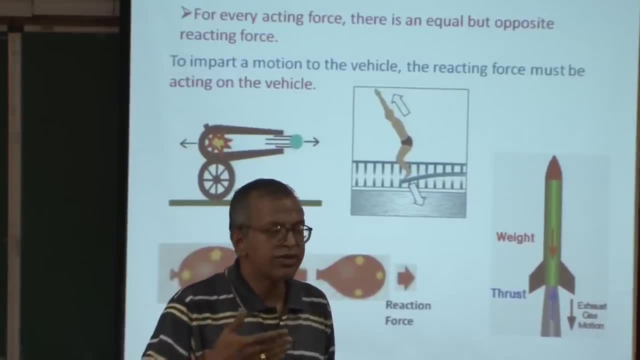 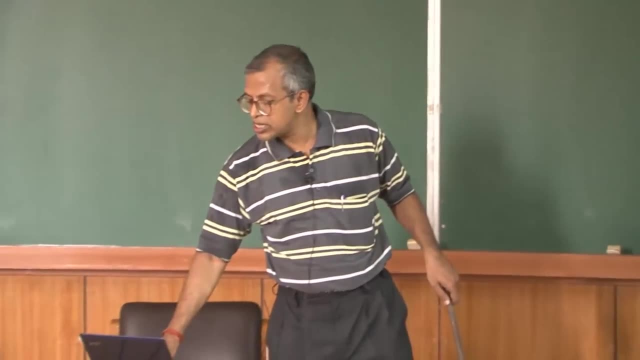 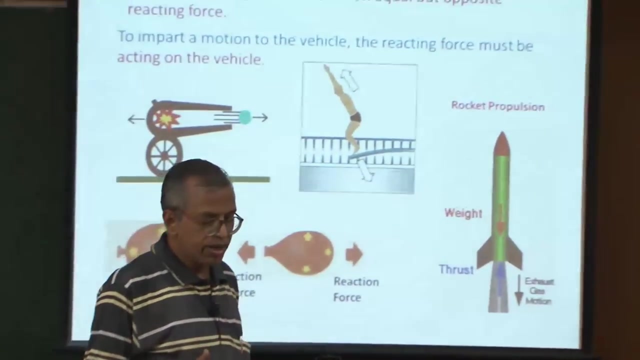 so that, and also the frictional forces, the drag, so that it will make a move. So this is the basic principle of the rocket propulsion. Now we will take this, This balloon, and look at what will be the gas turbine propulsion. I will take an example. 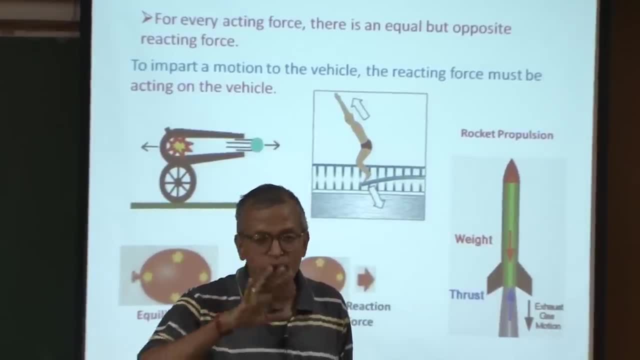 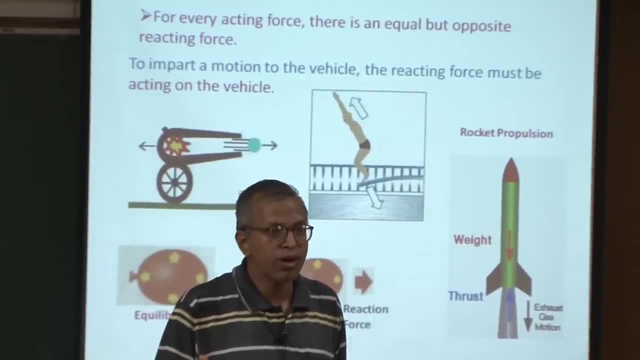 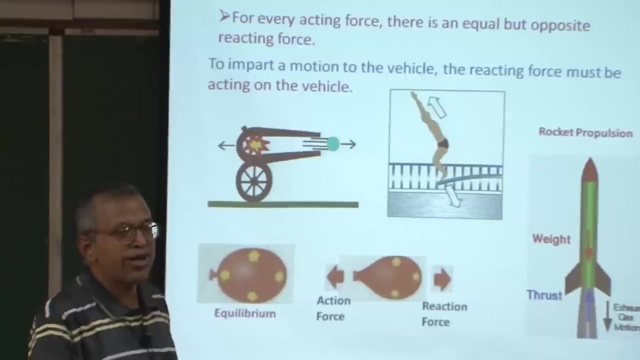 Now, before getting into that, I would like to ask you: we are talking about aerospace propulsion, but is there any occasion for us to think about life propulsion? that means we propel our life. You take a bath. from the bath to the death is the one journey in a 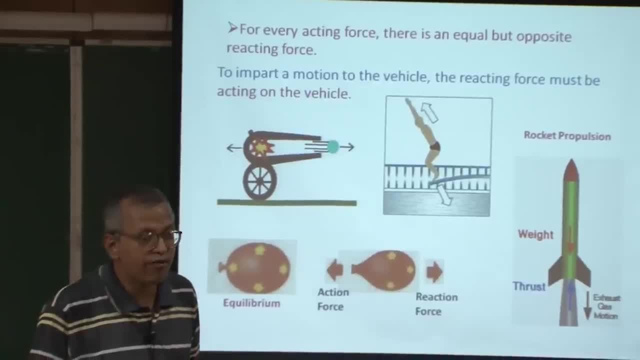 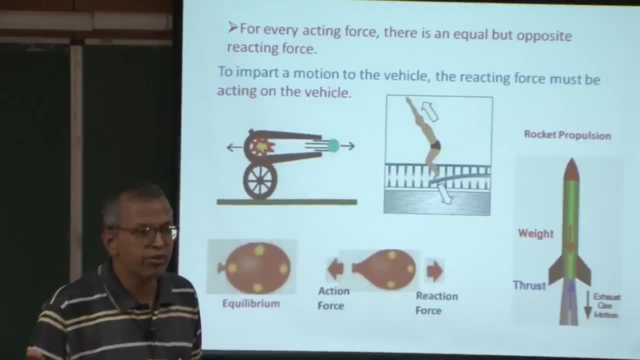 particular direction. Any of you have wonder any time how I will propel my life so that my life will be smooth and good. I can contribute, I can reach an excellent state. I do not think. some of you might be thinking, or some of you may not be thinking, and that is the main objective of all education.